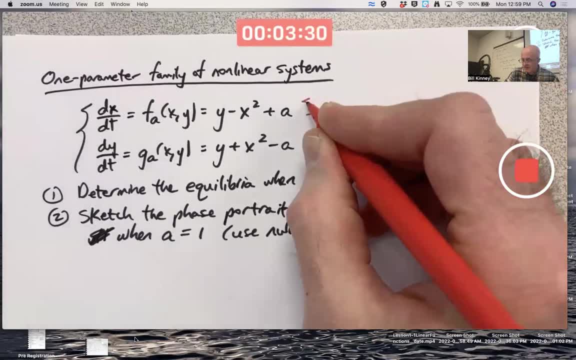 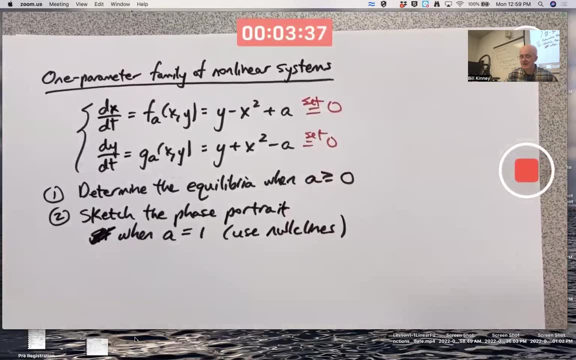 So first thing to do is set the right-hand sides equal to zero. When you set the dx to t equation equal to zero, you are essentially finding the x null cline. When you set the dy dt equation equal to zero, you're essentially finding the y. 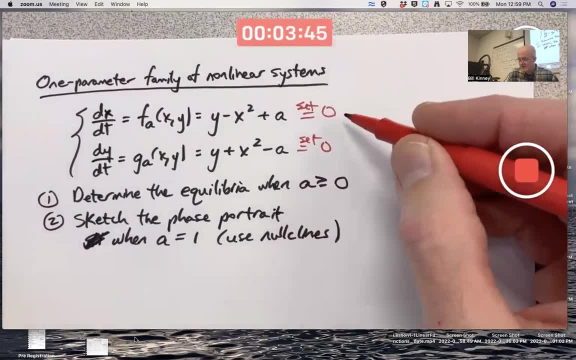 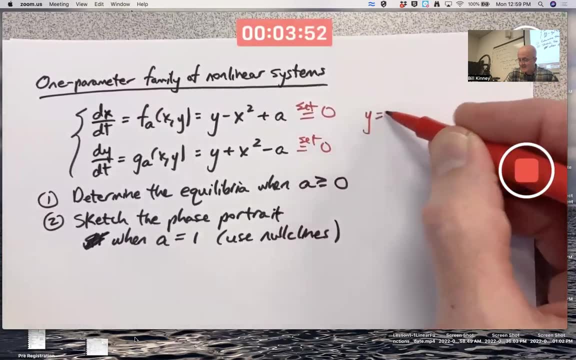 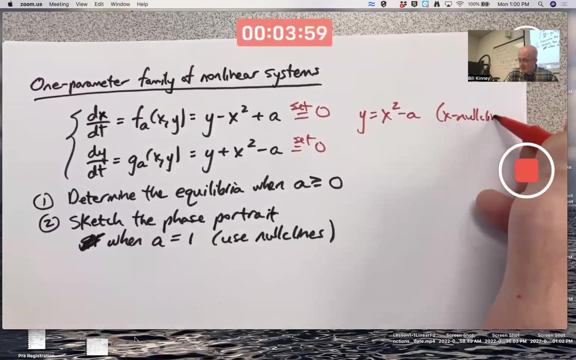 null cline. It's probably easiest to think about that in terms of y as a function of x in each case. So for the first equation, if you solve that for y, you get: y is x squared minus a. That's the x null cline. That'll be a parabola opening upward with y intercept. 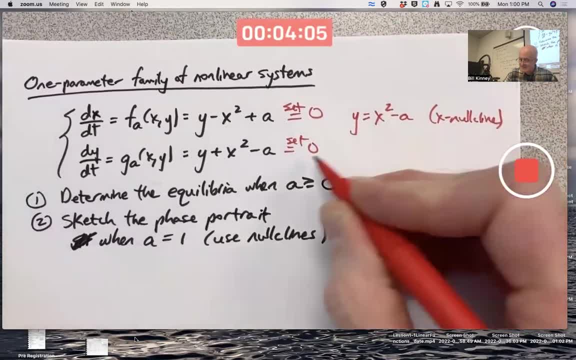 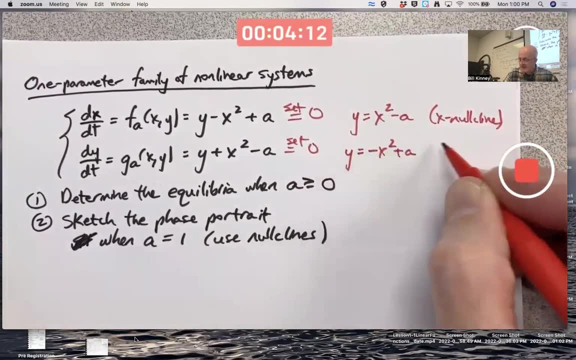 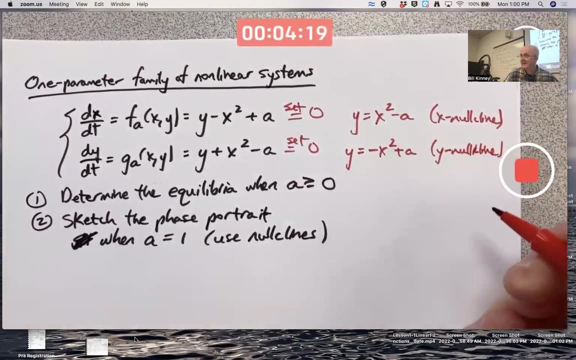 at negative a And looking at the dy dt equation solving for y, you get: y equals negative x squared plus a. That'll be the y null cline. It's the reflection of the x null cline across the horizontal axis, a parabola opening downward with the y. 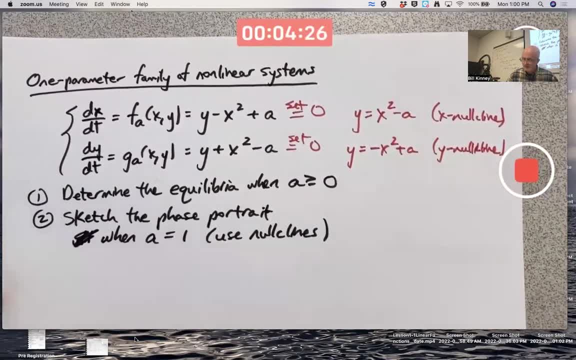 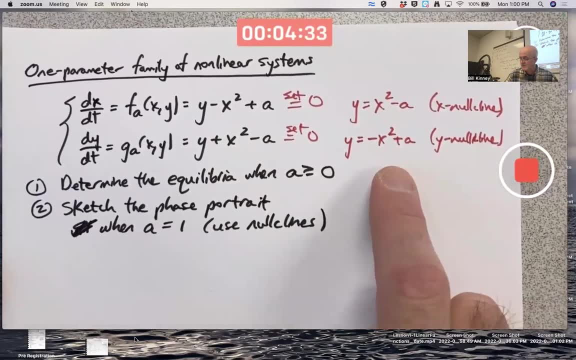 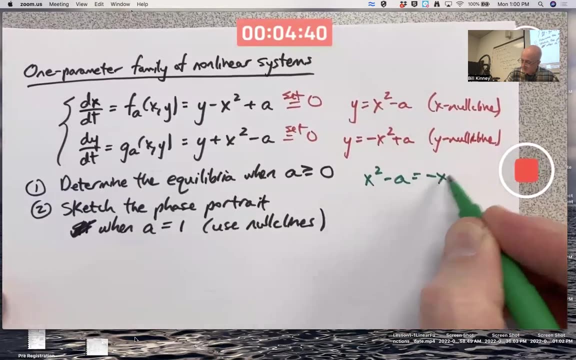 That's the y intercept at positive a. As far as finding the actual equilibrium points, it's where x and y null clines cross. So set these two things equal to each other. Set x squared minus a equal to negative x squared plus a and solve for x. Add x squared. 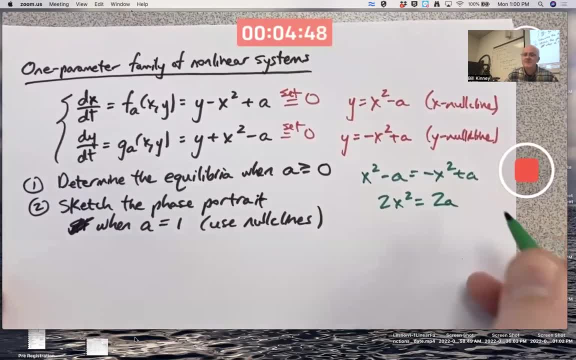 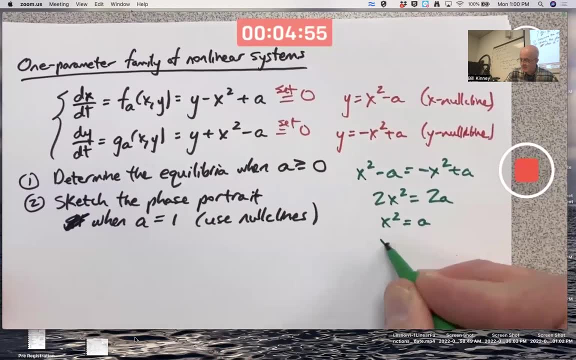 to both sides. Add a to both sides And you get 2x squared equals 2a. Divide both sides by 2x squared. Take the plus or minus square root of both sides. The x coordinates of equilibrium points are at plus or minus the square root of a. To find the y coordinate, plug those back. 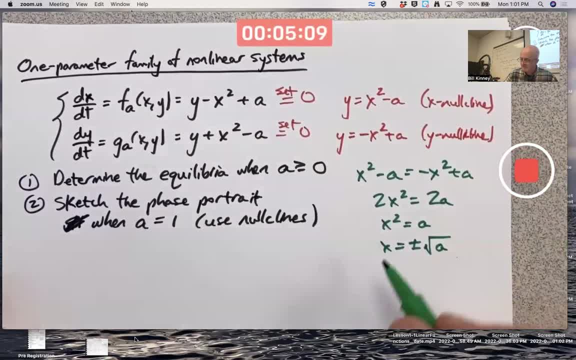 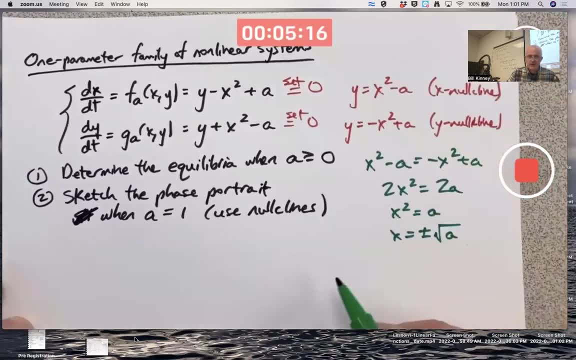 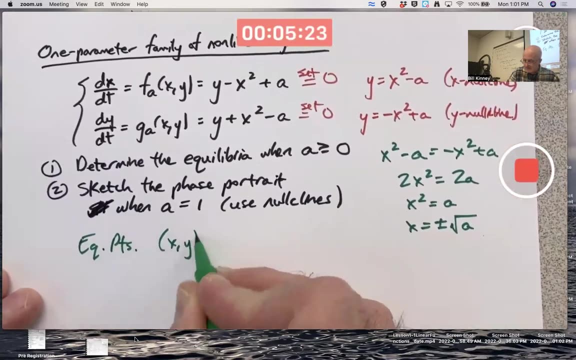 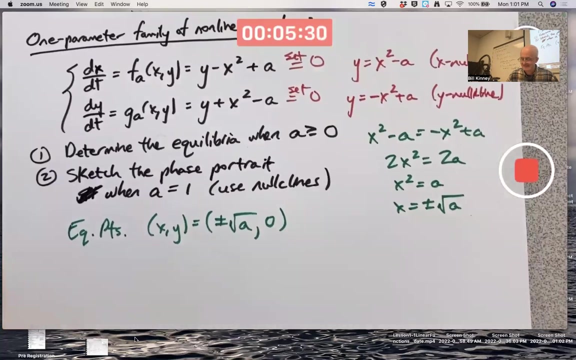 into either equation and you get y equals 0. Square that You'll get a. a minus a is 0. Also negative: a plus a is 0. So your equilibrium points, the x coordinates, are at plus or minus the square root of a comma 0. They are on the x axis When a is 1, that's. 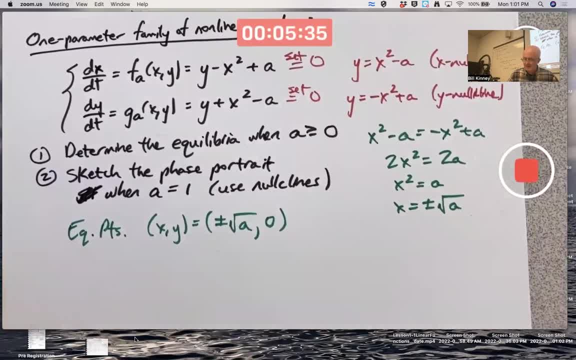 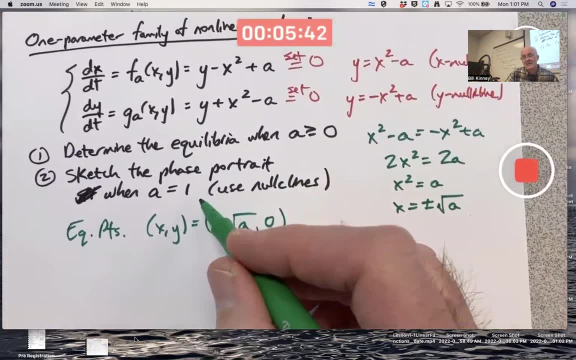 plus or minus 1 comma 0.. Let's try to draw the phase portrait. I could say a is 1, but really perhaps the phase portrait looks basically the same. for any positive value of a, The location of the equilibrium points is going to change. 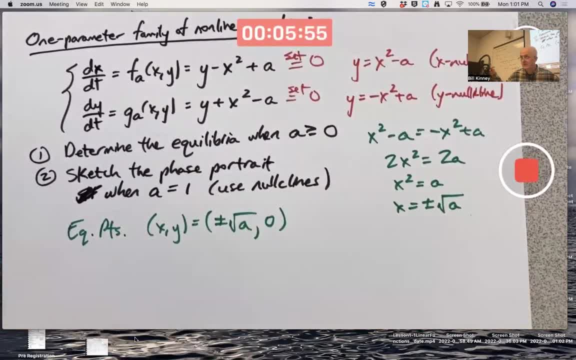 Clearly, as a increases they will move further away from the origin. Does that make sense? Because that's going to get further away from 0 as a increases. But maybe the picture basically looks the same. Let's see if it seems reasonable to assume such a thing, at least If a is. 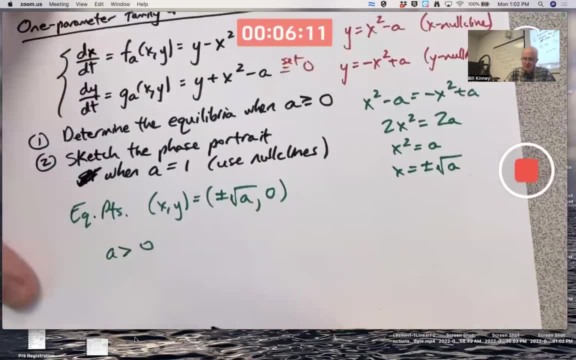 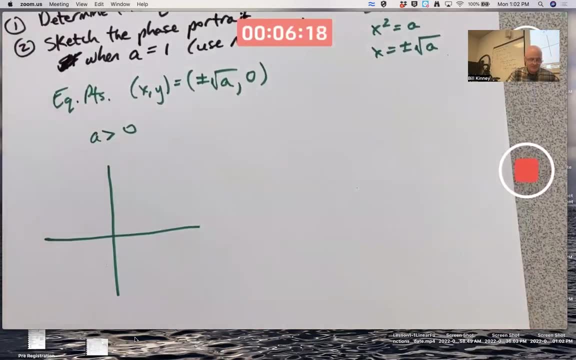 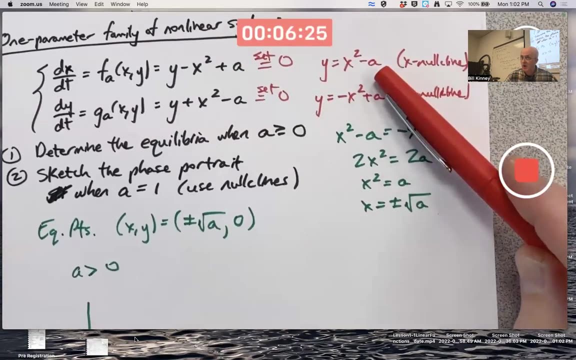 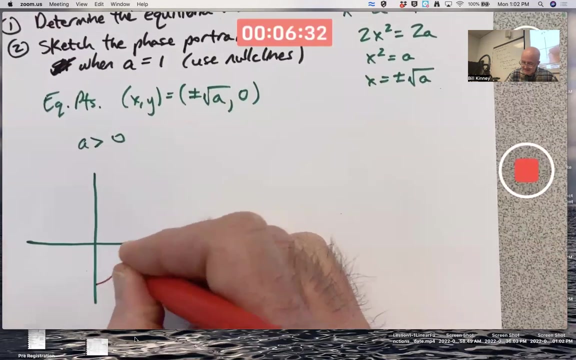 positive. what does the phase plane look like? Draw the no-clients to help you. The x no-clients remember, was y equals x squared minus a. a parabola opening upward y intercept at negative a. So the x no-clients looks about like this: It's an x no-clients, so you got. 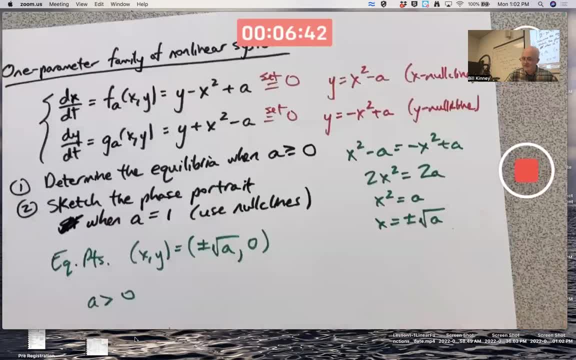 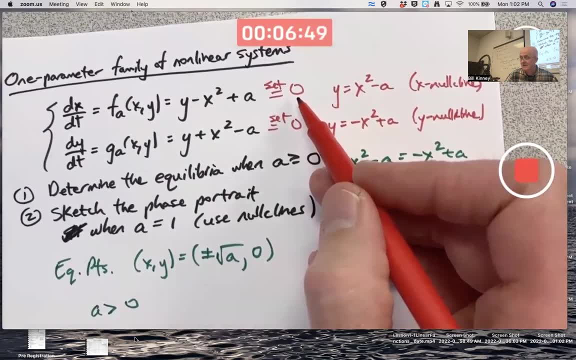 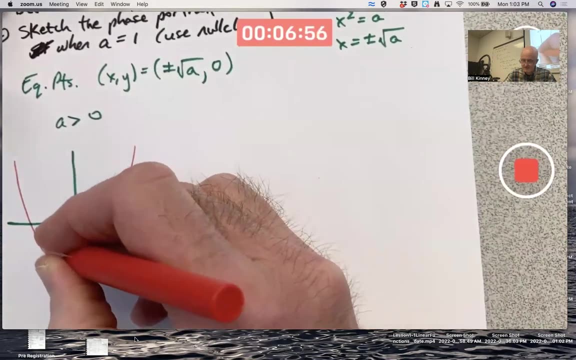 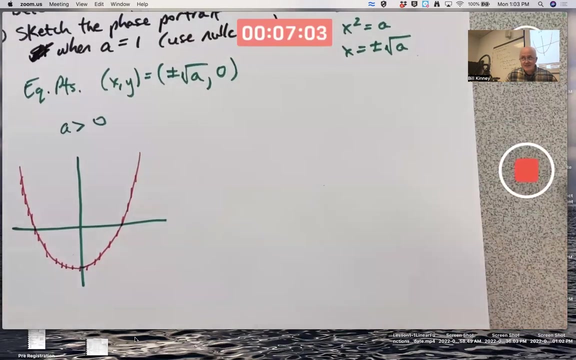 to cross that with 0, dx, dt 0, first component of velocity vectors in the vector field, You got to cross it Vertically, Make a bunch of little vertical lines. It's not a straight line solution, It's not even straight. It's not a curve solution, It's not a solution at all. It's just showing. 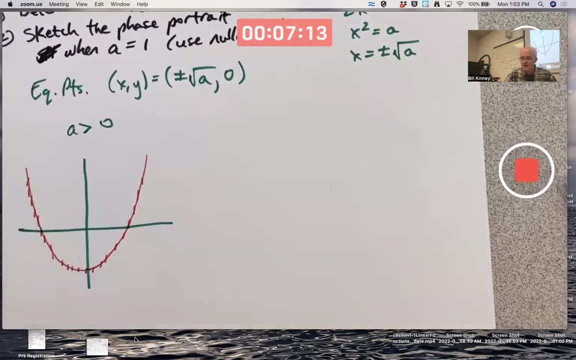 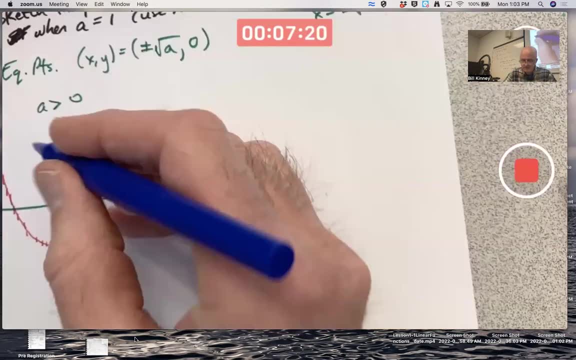 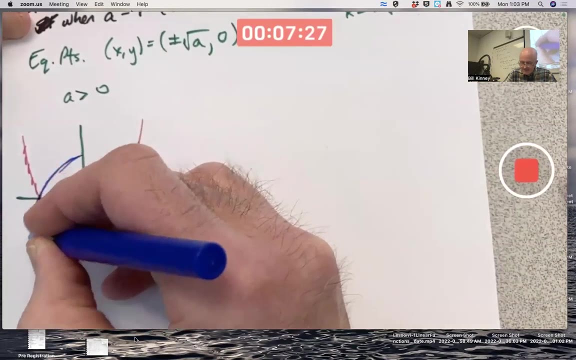 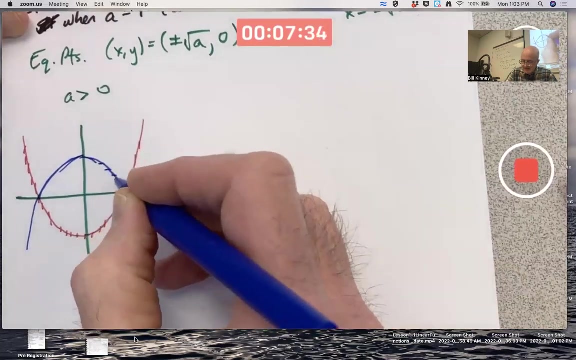 you how the solution curves cross that line- The y no-clients is the reflection of that- across the horizontal axis downward, pointing like that About, like this. And yeah, where they intersect by symmetry, it's got to be on the x axis. You're going to cross that horizontally. 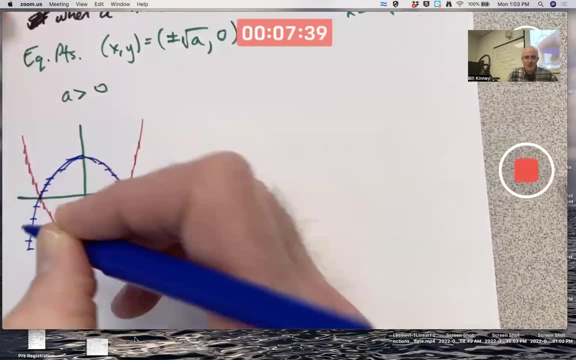 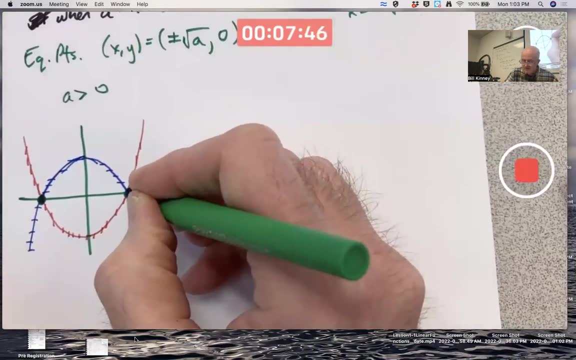 And where x and y no-clients touch. that's equilibrium points here and here I saw many of you got this far. But then the hardest parts Here From this perspective: Here, different points across the horizontal axis, So some of which are at x and some are at 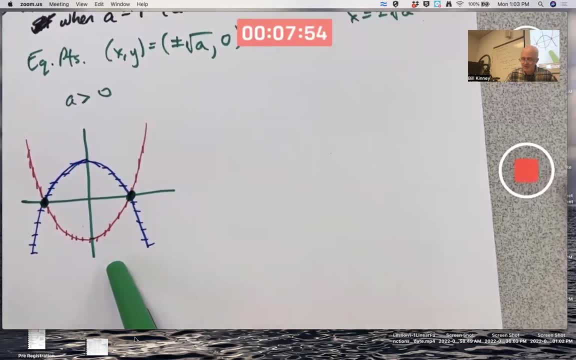 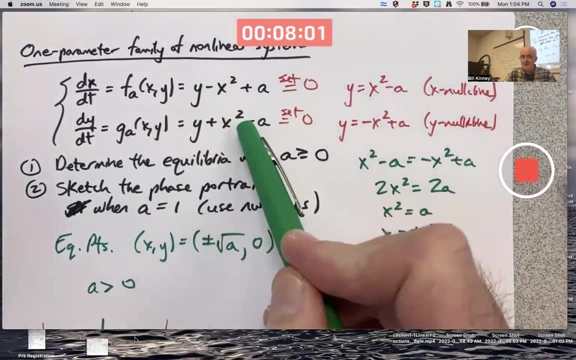 y. And then we've got to try to know where those Selbstman mientras pass there At either模 pins. But then the hardest part is drawing the phase portrait. after that point, Think about the signs of these things. the right-hand sides. 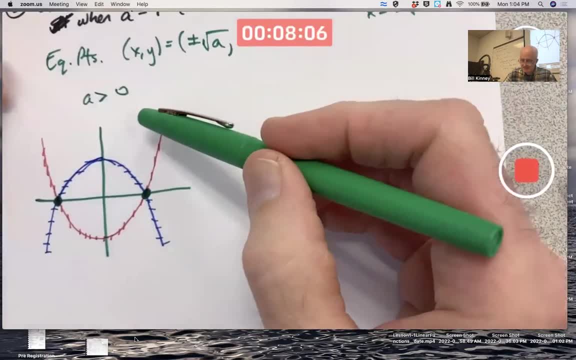 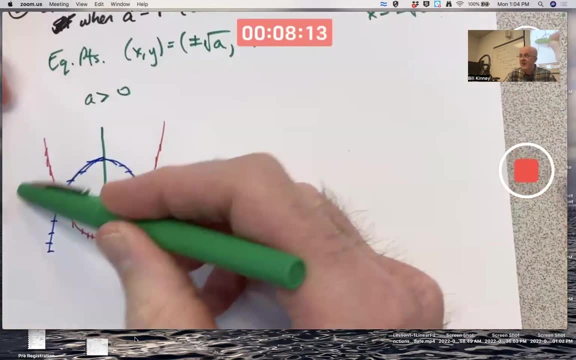 in how many different regions, The regions in the plane separated by these noclines? There's one up here, there's one in here, there's one down here, one over here, one over here. Five regions to think about signs of dx, dt and dy dt. 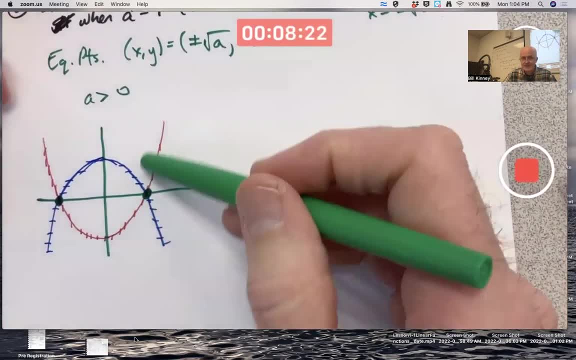 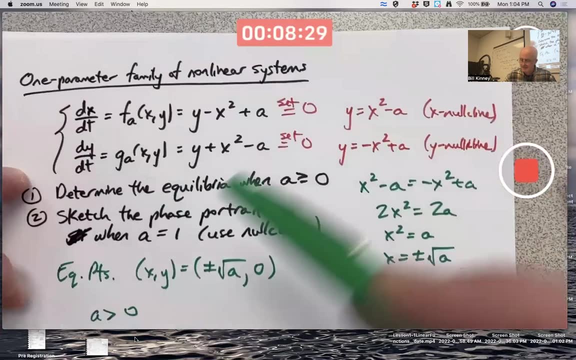 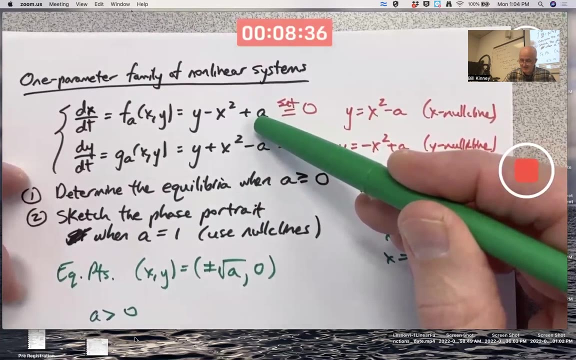 Actually you can focus on each one individually. Again, the red one is the x nocline. The vector field is 0 along there. Think about this: Is that positive above that red parabola, or negative? When a is positive, you could try a test point. 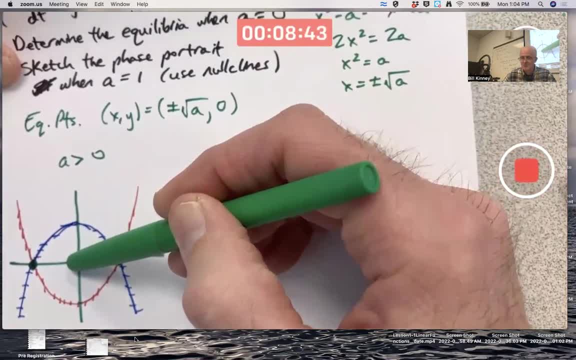 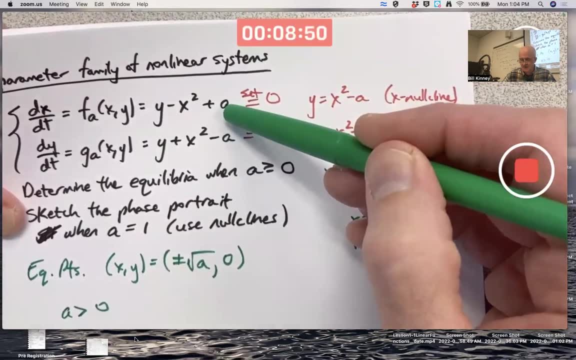 like the origin. for one thing You could try Plug in: x is 0, y is 0, you just get a And a is positive, So that's positive. When you're above this red curve, solutions have to be going to the right. 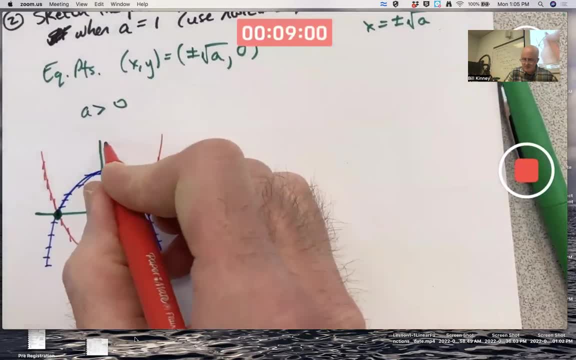 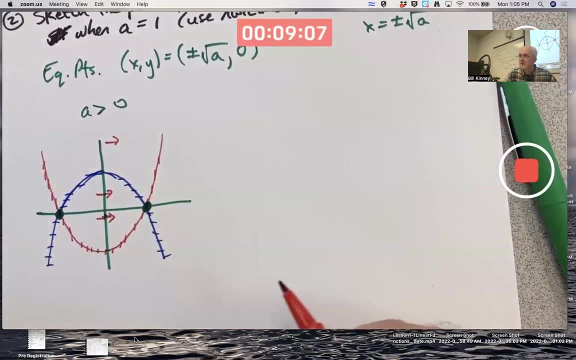 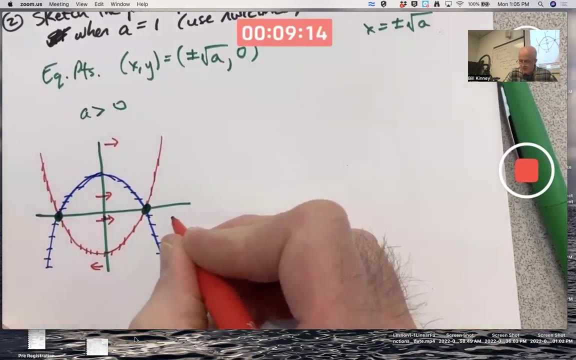 The x dt has to be positive. So the rightward pointing in this region and also rightward pointing in this region, those are both above the red curve, Downward pointing, below the red curve Down here, over here, excuse me, leftward pointing. 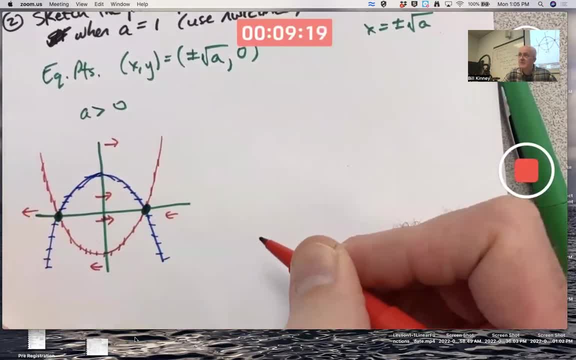 The x, there is a positive. There was a left SEC T there The x, there is a positive. And they are both above a red curve, Downward, pointing below a red curve. below the red curve, We're focused on dx, dt. 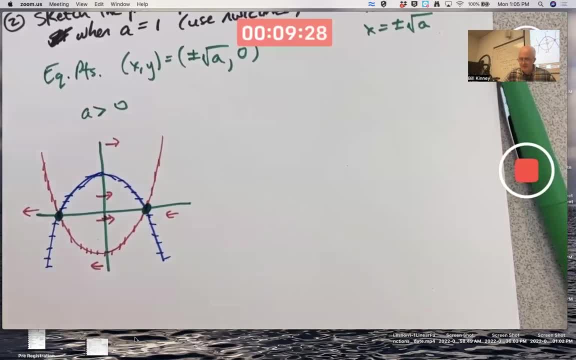 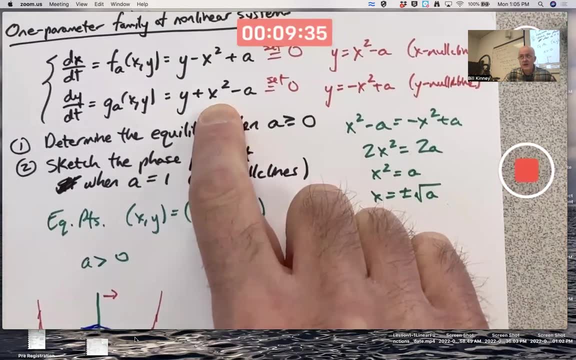 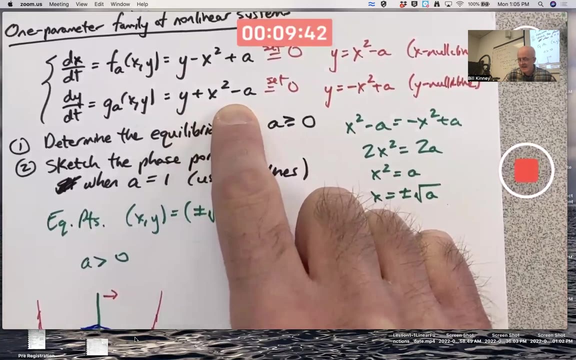 So we need to think about: do solutions go right or left? dy dt think about the sign positive or negative of that. Again, you could plug in the origin as a test point. Plug in: x is zero, y is zero. you get zero minus a is negative a. 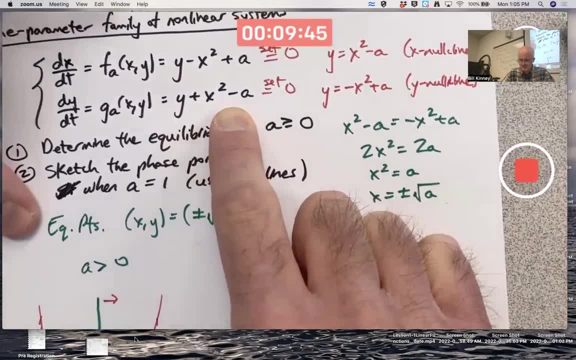 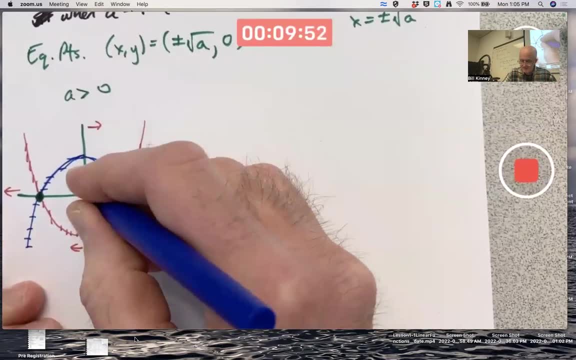 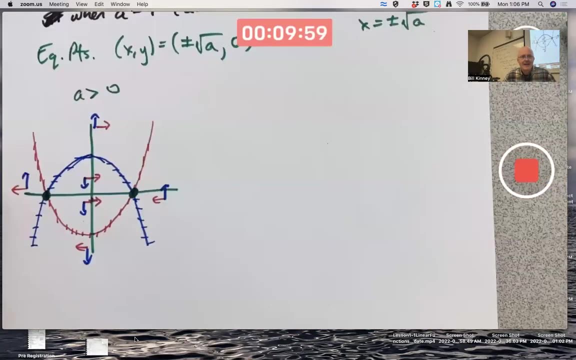 And if a is positive, that's negative. So at the origin, dy dt is negative. When you're below the blue curve, dy dt is negative, And when you're above the blue curve, dy dt is positive. Now try to draw solutions, the very hardest part. 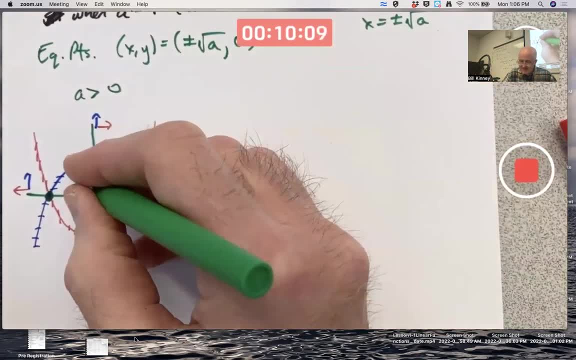 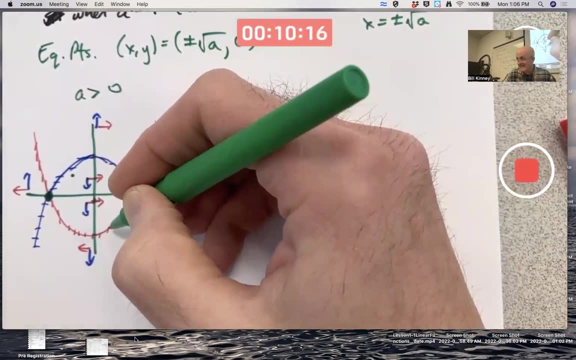 Pick, sort of like a random initial condition. Oh, I don't know, maybe in here, to start with, These arrows indicate you've got to go to this direction to the southeast. How far will it go? That's hard to say. 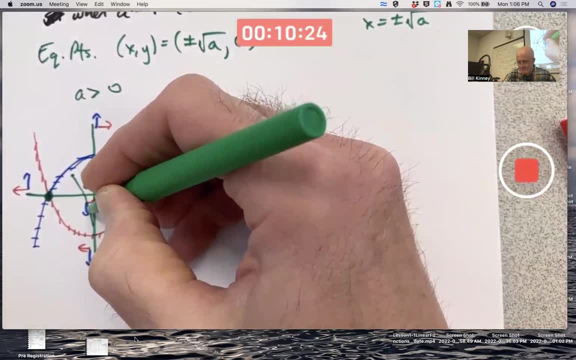 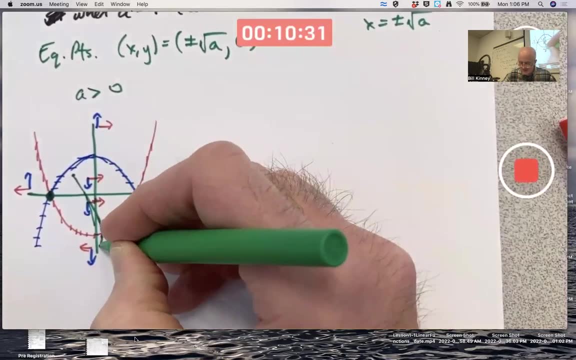 but it will cross the x and y-line somewhere. Okay, I've drawn that one to make it look like it's going to cross on the y-axis, but maybe it goes over here. And then you got to go to the southwest and you go out this way: 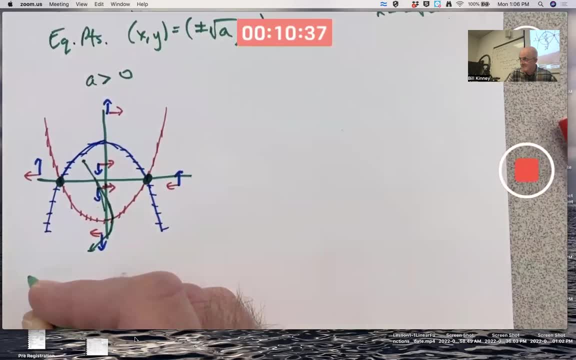 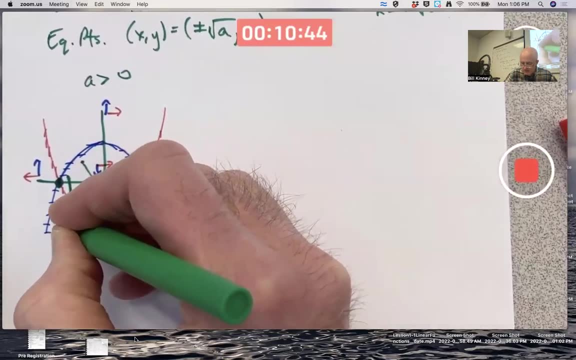 And probably at some point you're going to cross the blue parabola again. If we started closer to this equilibrium point, maybe it's more clear, More clearly. crosses the blue parabola right about here. Then you're going to the northwest. 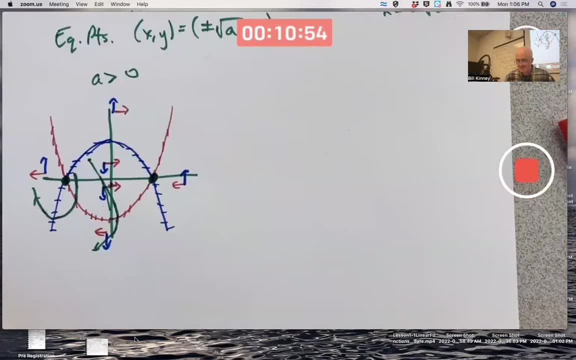 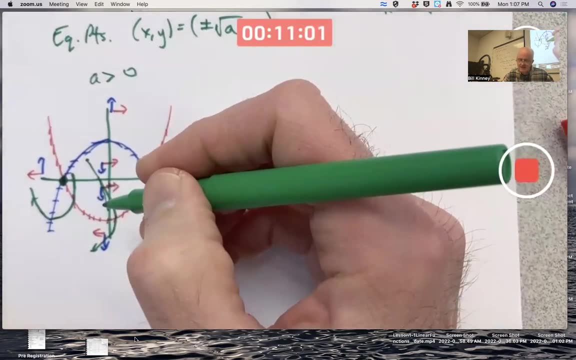 It can't possibly cross the red parabola again, right? Because if it did, it would have to at some point. Well, excuse me, I guess it could Never mind. I said that wrong If it was close enough here. 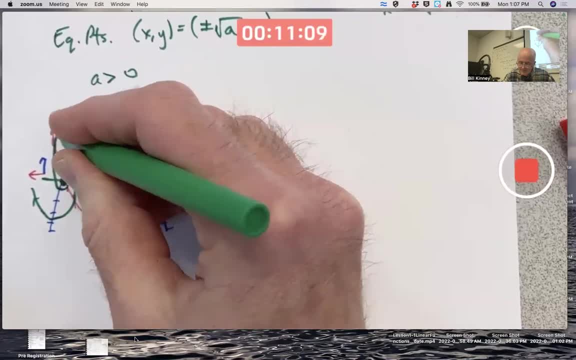 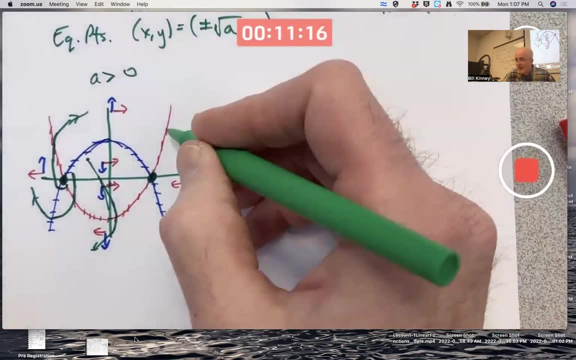 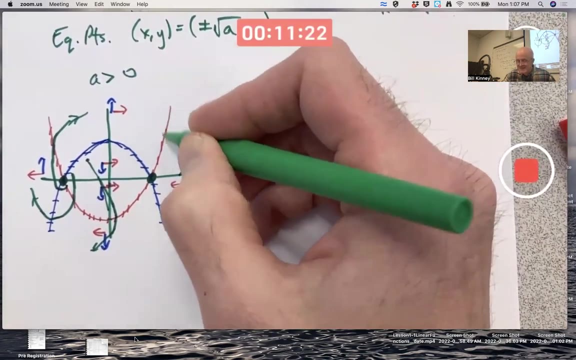 certainly it's going to cross the red parabola like that before going to the northeast There. it can't possibly cross the red parabola over here, Because if it did, it would have to be going to the southeast there and it can't. 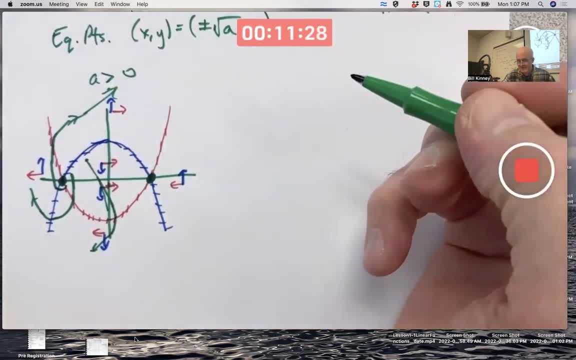 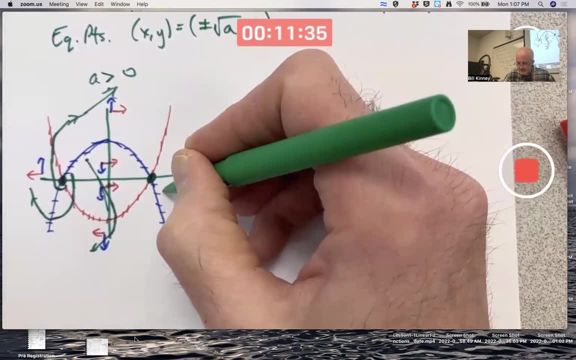 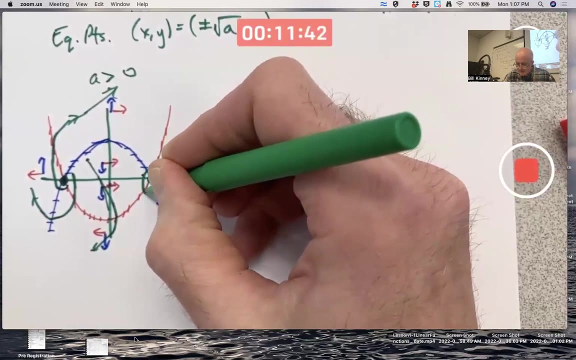 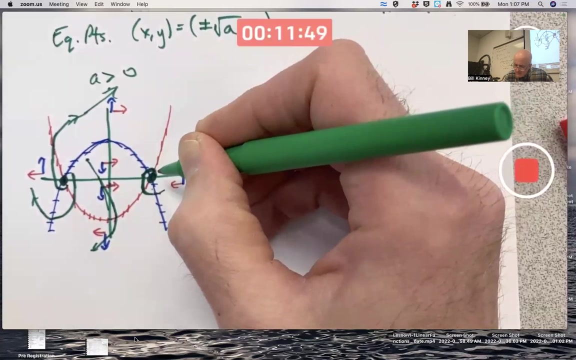 It's got to continue going to the northeast here, Pick some other initial conditions, maybe one over here. Symmetry probably is going to come into play. I'm not doing a very good job here. Cross that horizontally, Oh no, no, no, I'm doing a really bad job, sorry. 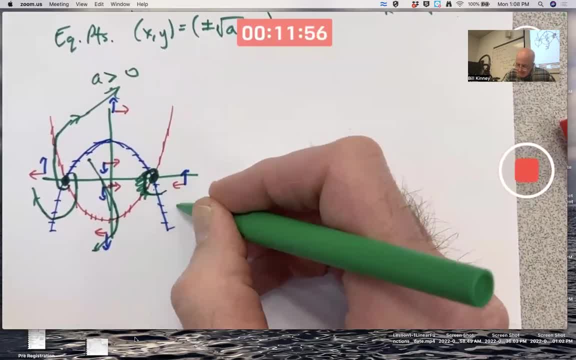 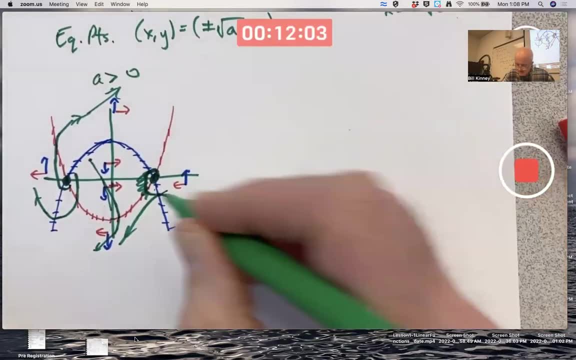 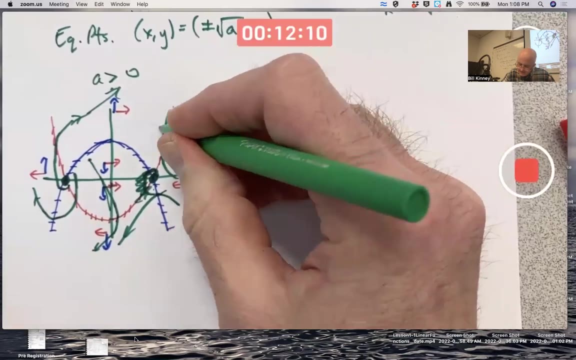 Ignore that easy to make a mistake. Go to the northwest here before crossing. Then you're going to the southwest. Ignore this Here. you'd cross this way before going to the northeast. It should make some intuitive sense by continuity. There's got to be some solution. curve. 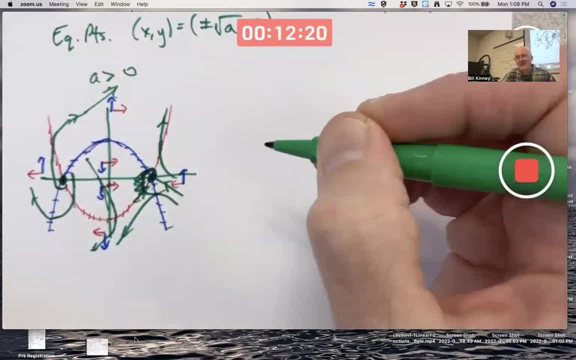 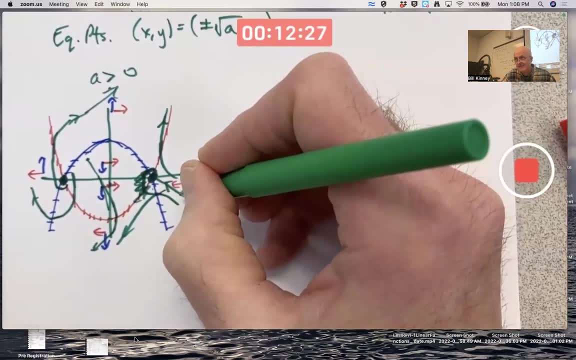 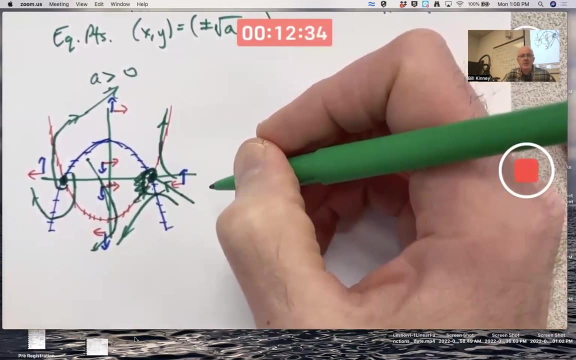 that heads straight toward that point, Maybe not actually on a straight line. I know I said the word straight, but it doesn't necessarily have to be a straight line. It's probably not. Guess symmetry is not coming into play as much as I was initially thinking here. 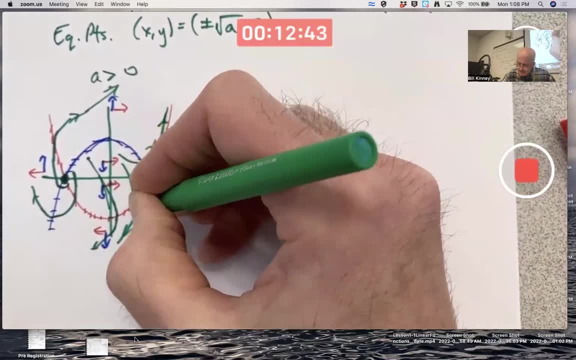 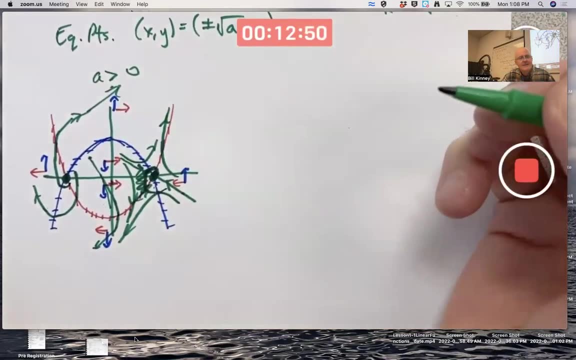 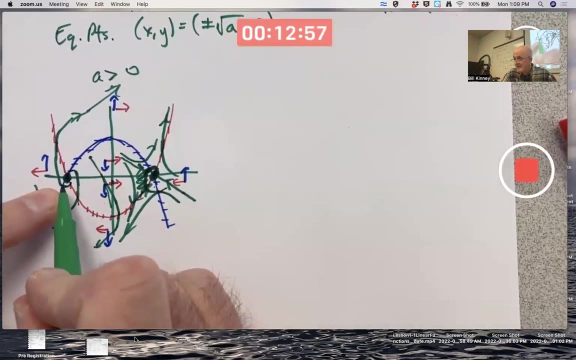 Drawings in some other solutions here, There's got to be one that's going toward the equilibrium point. this way You start to get a little feel for what's going on. It looks like this point right here. Look at it with me here. 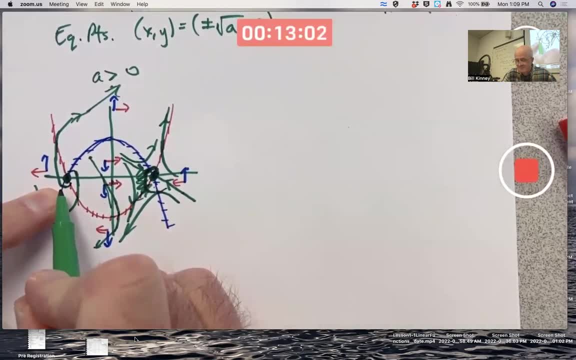 That looks like some sort of spiral source, doesn't it? And this point looks like some sort of saddle point. But how do you know? Is there a way to know for sure this is a saddle point? Is there a way to know for sure? this is a saddle point? 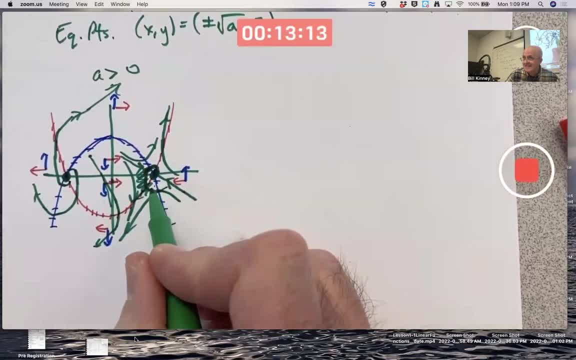 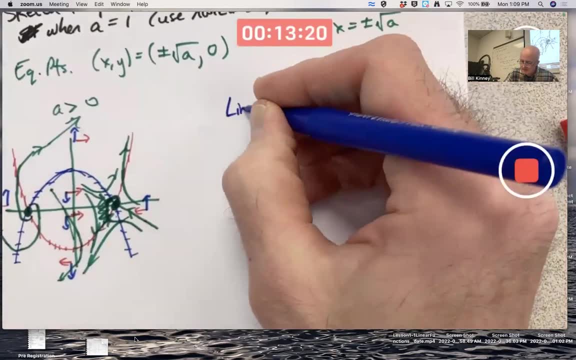 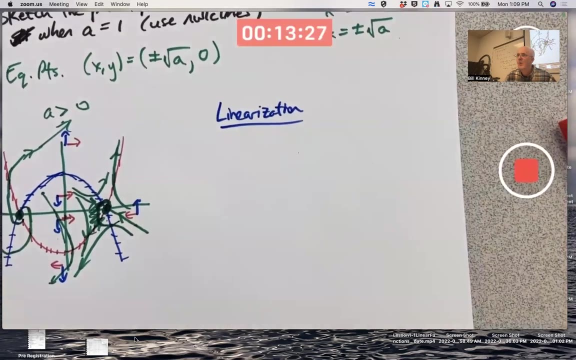 Is there a way to know for sure? this is a spiral source and this is a saddle point. There actually is. That's called linearization, where you try to get rid of nonlinear terms, essentially in the differential equations on the right-hand sides. 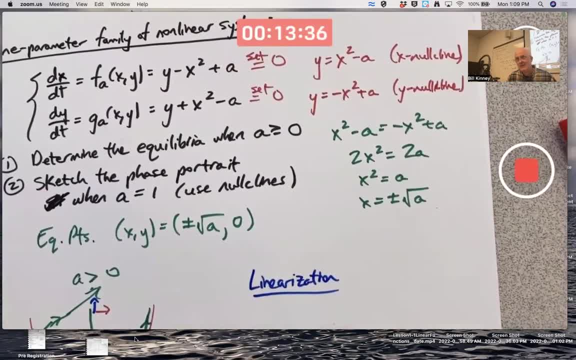 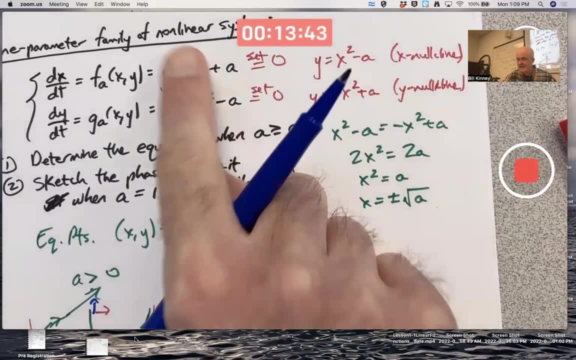 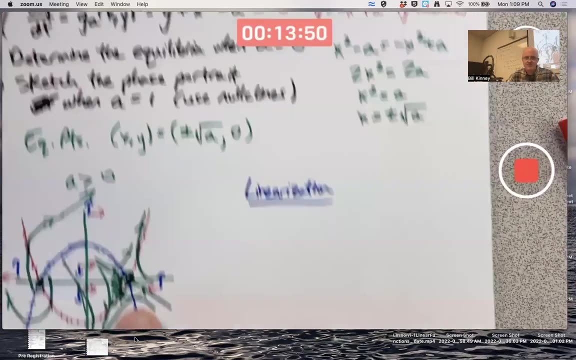 However, I said, get rid of nonlinear terms, with the caveat that you only do that in the most obvious way, like deleting those x squared terms when your equilibrium point is at the origin. Our equilibrium points are not the origin. unless a is zero, then they merge. 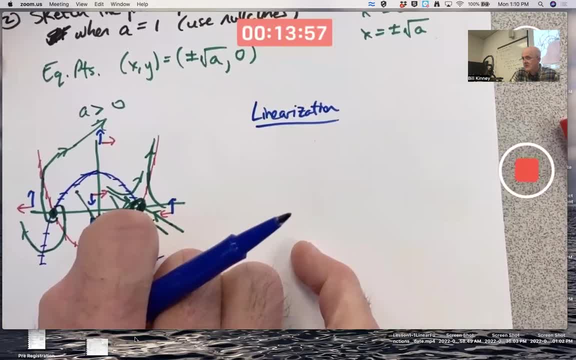 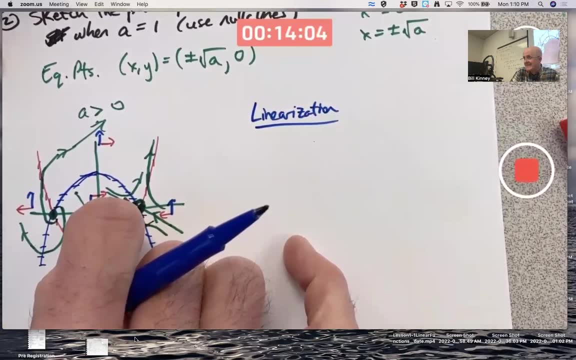 That's why a is zero is a bifurcation value. As a approaches zero, these two equilibria merge into one equilibrium point at the origin. And then, when a is negative, they have annihilated each other, And then, when a is negative, they have annihilated each other. 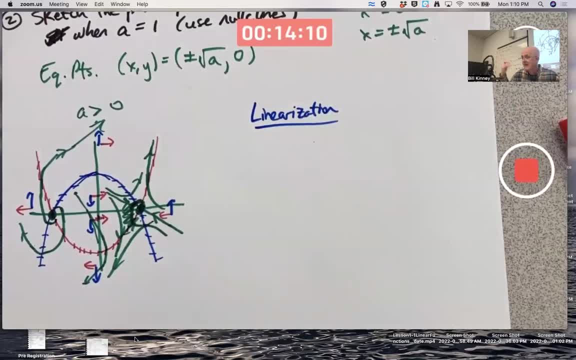 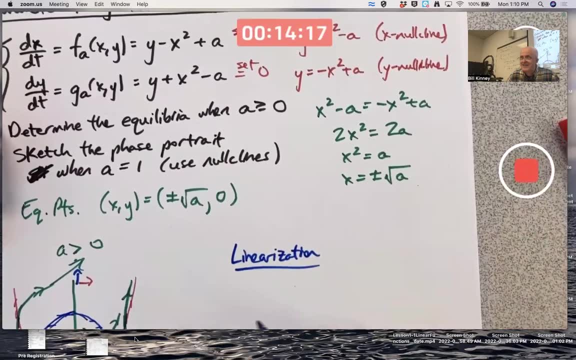 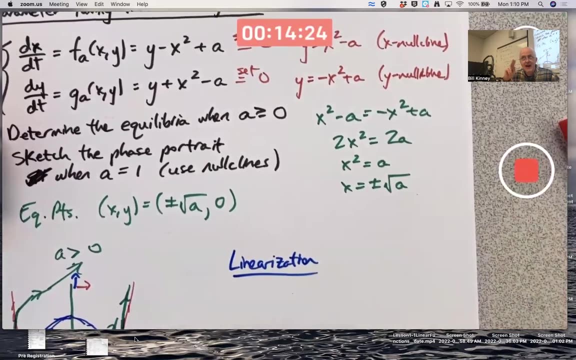 There's no equilibrium points when a is negative. Yes, we want to throw away nonlinear terms, but if the equilibrium points are not at the origin, that's tricky. There's two ways to approach it. The book talks about both methods. I also talk about both methods in the lectures. 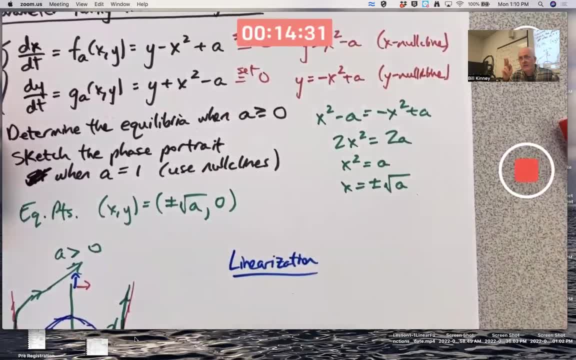 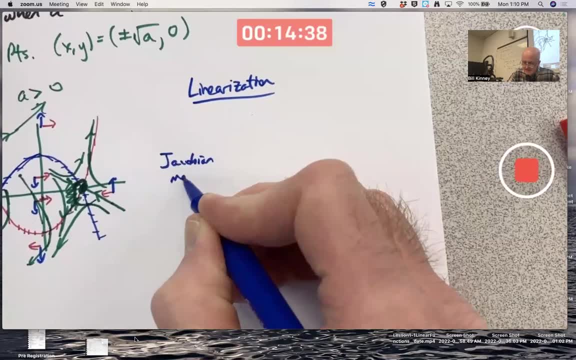 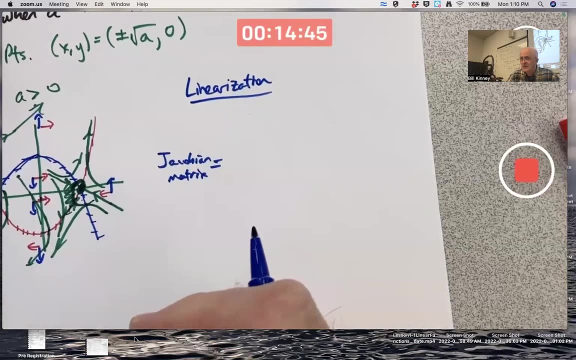 The simpler method is to use something called the Jacobian matrix. Jacobian matrix- Anybody in here had multivariable calculus- A few of you in the back, okay. yeah, You probably heard about Jacobian matrices and multivariable calculus. 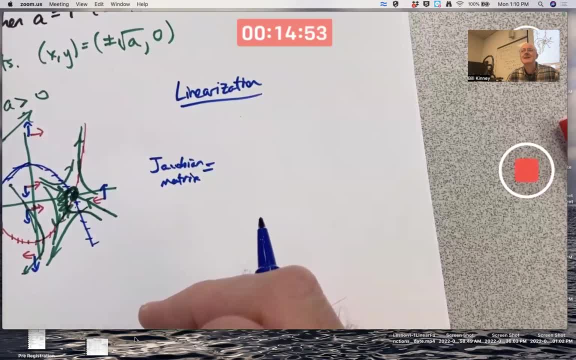 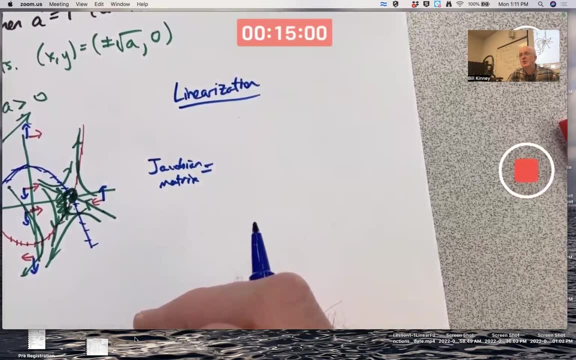 They're showing up here again. The purpose is different. In multivariable calculus the purpose is to use Jacobian matrices in the determinants to do change of variables, general change of variables for double integrals, triple and triple integrals. And then you can use Jacobian matrices in the determinants to do change of variables- general change of variables- for double integrals, triple integrals. And then you can use Jacobian matrices in the determinants to do change of variables- general change of variables for double integrals. 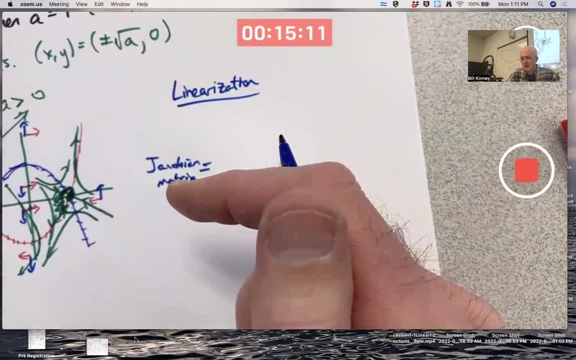 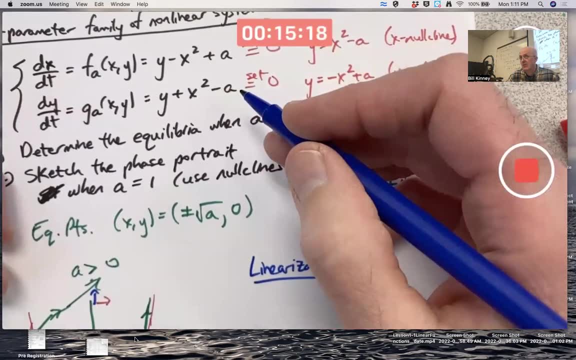 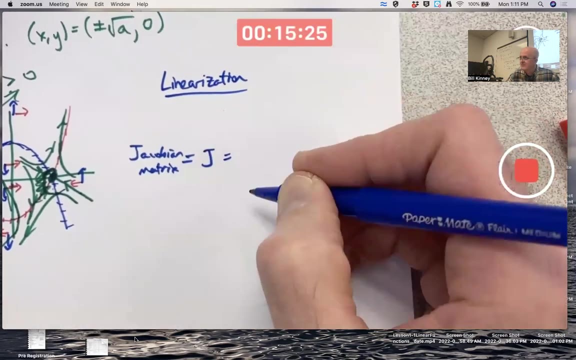 Here the purpose is different. The purpose is to do what's called linearization, to essentially try to approximate this nonlinear system with a linear system near the equilibrium points. I call J in honor of Jacobi, though other people call it D in honor of derivative. 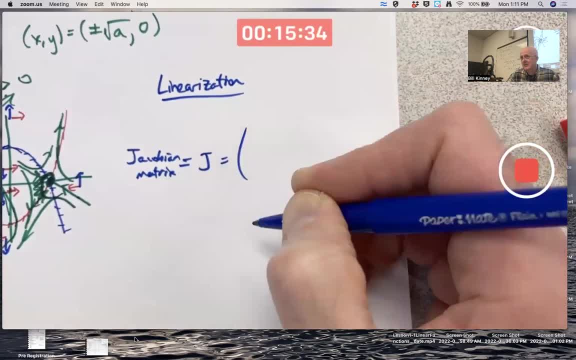 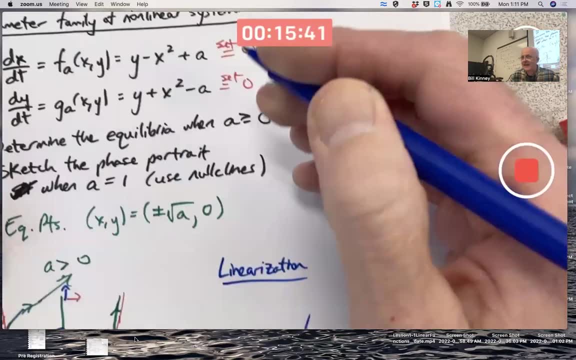 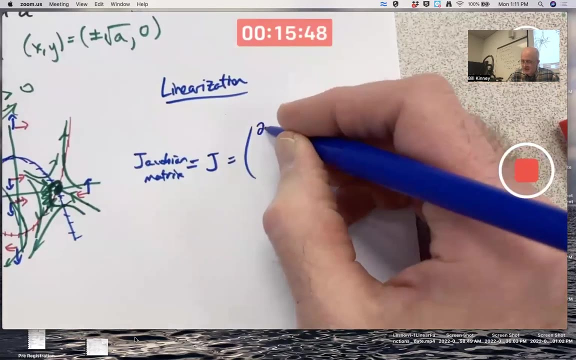 Derivative is not a person's name but, because it is kind of a derivative, it's a matrix whose entries are the partial derivatives of the right-hand side functions with respect to x and y, Upper left entry is the partial of the first component. 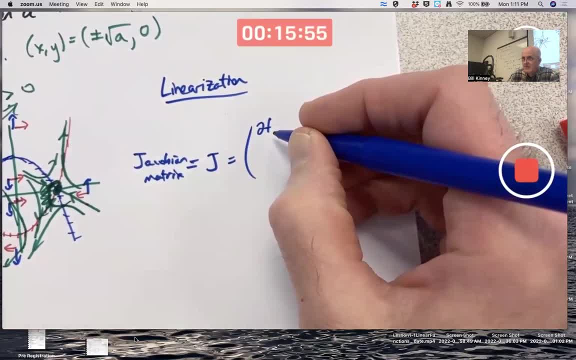 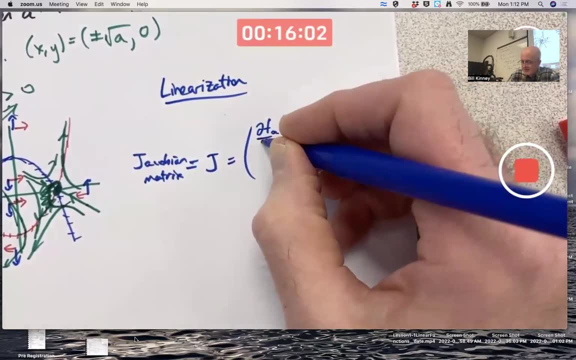 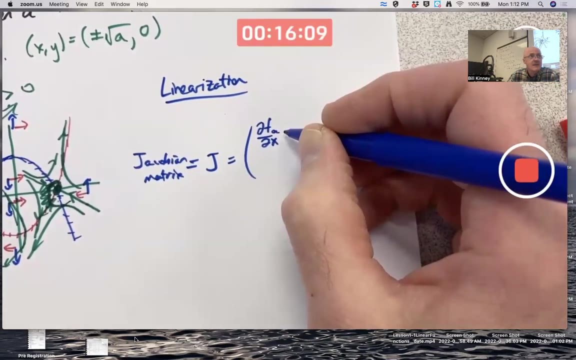 of the vector field, little f. I won't bother with the subscript a. I could. no, maybe I should. With respect to the first variable, you won't always have a parameter there. We do here. Let's have it quiet here, please. 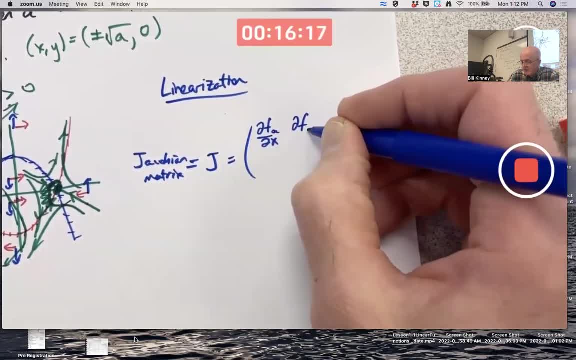 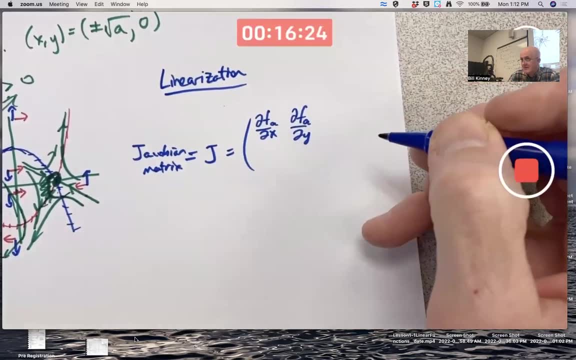 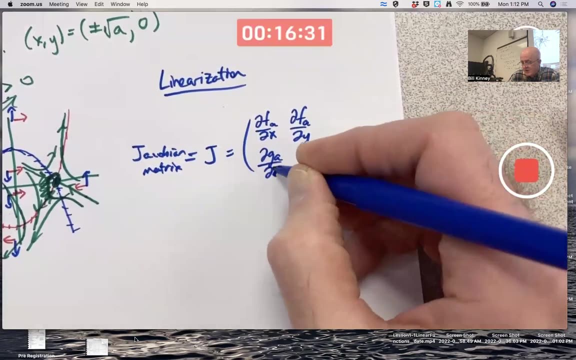 This upper right entry is the partial of that first component. with respect to the second variable, Again, the a is just the parameter here. I was tempted to not include it at first, but I'm including it. Lower left is the partial of the second component. 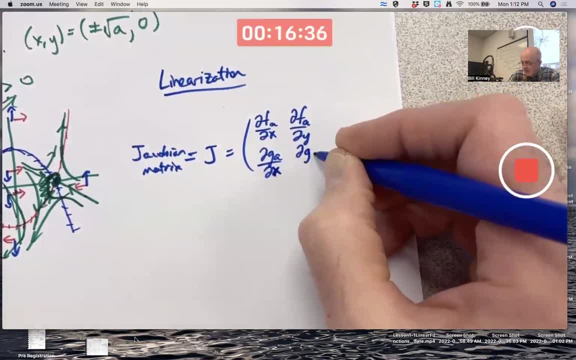 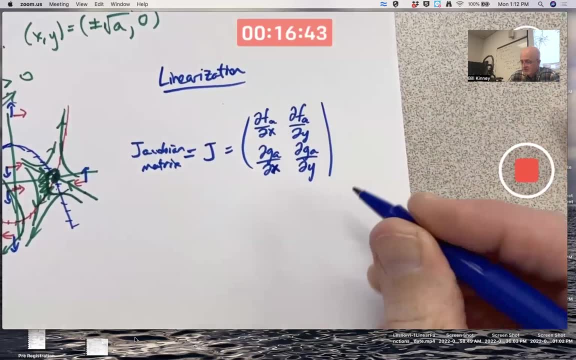 of the vector field with respect to the first component. So this is the first variable, and lower right is the partial derivative of the second component with respect to the second variable. This is called partial derivative notation. These curvy things are essentially fancy Ds. 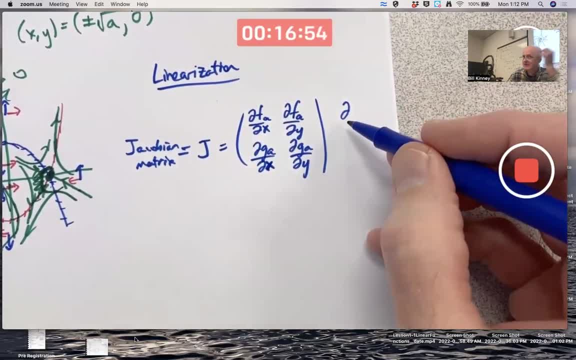 The only reason to use a fancy D in this context is just to emphasize mentally: oh, my functions depend on more than one variable And so that's just sort of a way to remind yourself of that. You could use R ordinary d's. don't read too deeply into this. it's just a convention. 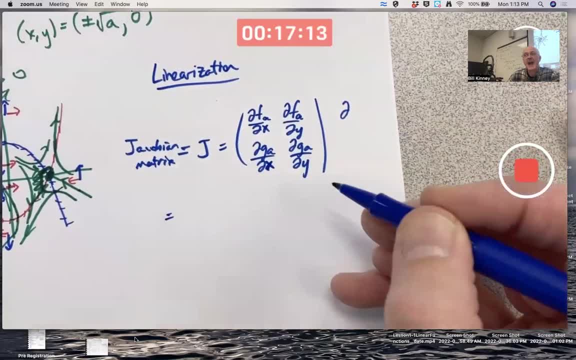 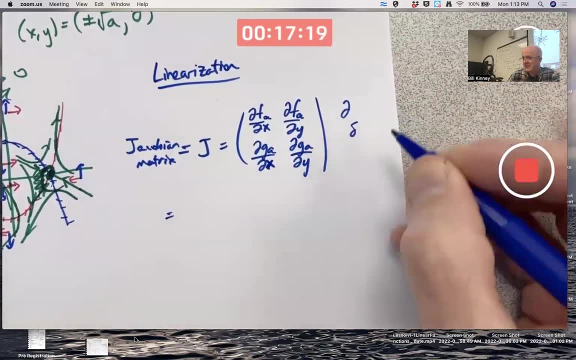 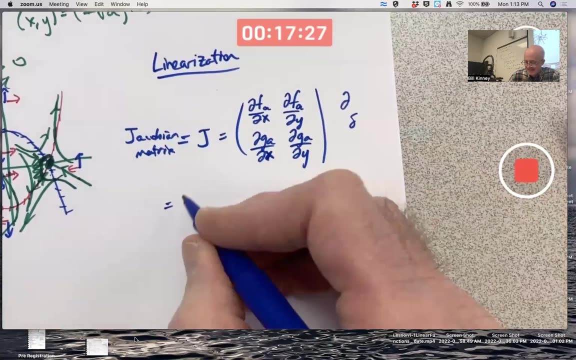 it gets even extra strange in some physics classes because sometimes you'll use deltas instead of d's and it's like weird, why? why are you using deltas sometimes and these other times and stuff? it's confusing, right? it's just not a big deal, don't worry about it. 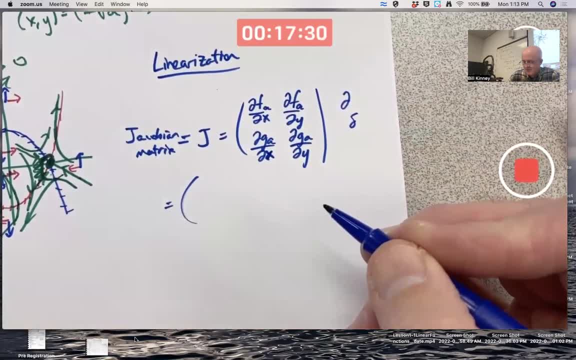 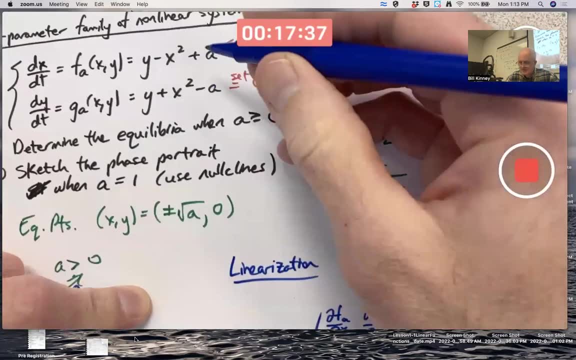 it's confusing because different people have different preferences with those things. okay, so how do you take partial derivatives? you just treat with respect to x, you just treat y as a constant and of course, a is a constant. so you differentiate this with respect to x. you're just. 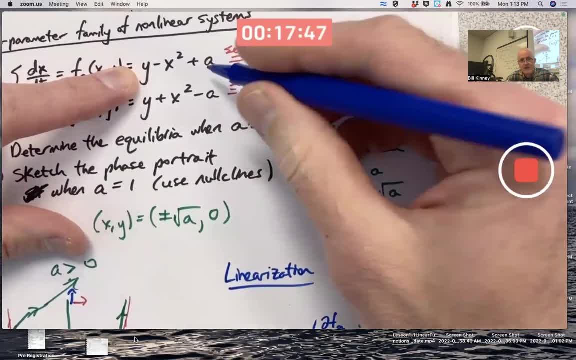 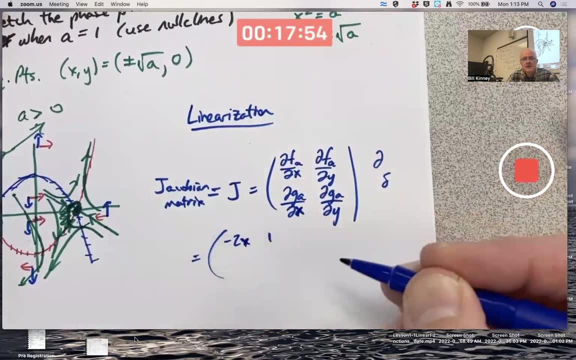 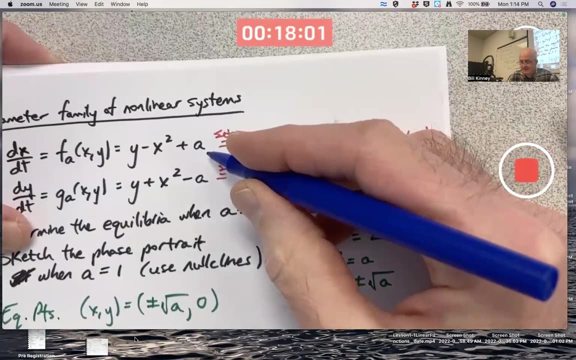 going to get negative 2x. differentiate it with respect to y, you just get one negative 2x and one right. differentiate this with respect to x. treat the y and a as constants. it's negative 2x, x. differentiate it with respect to y, you get one. something kind of similar happens. 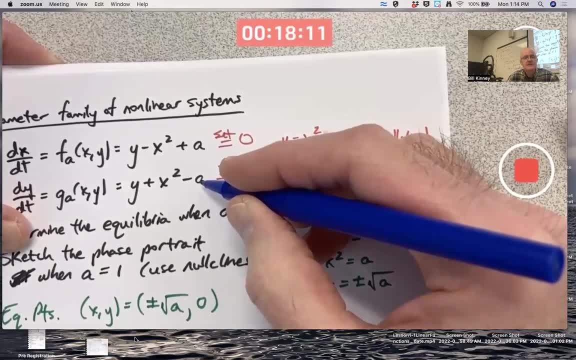 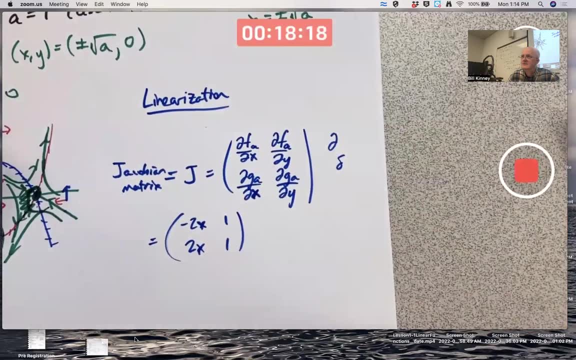 with this one, except the derivative with respect to x is positive 2x. there's your general jacobian matrix. it's a function, a matrix valued function. plug in a point x, y, you get a matrix. weird. well, we do weird, lots of weird things in this class, but 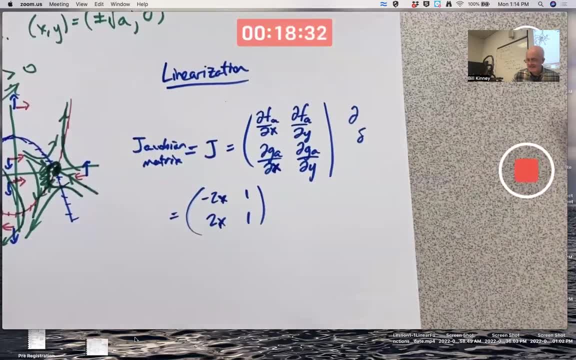 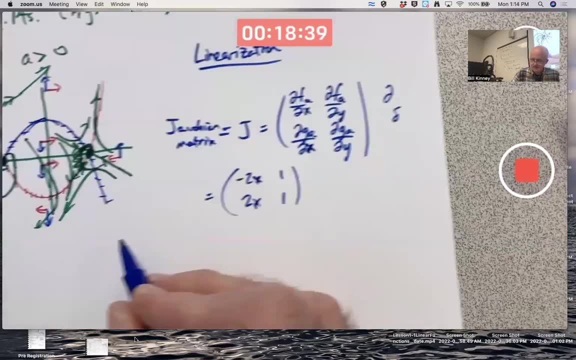 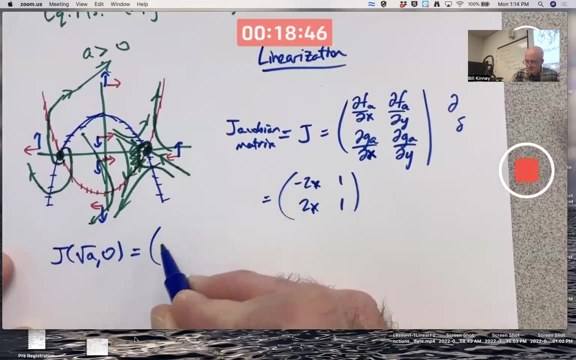 there it is. what do you want to do with it? you want to plug in the equal of room points into it. j of square root of a comma. zero is what? replace x with square root of a. replace y with zero where there are no y's. so you don't have to. 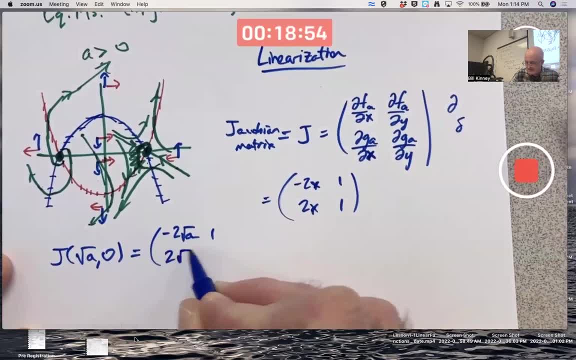 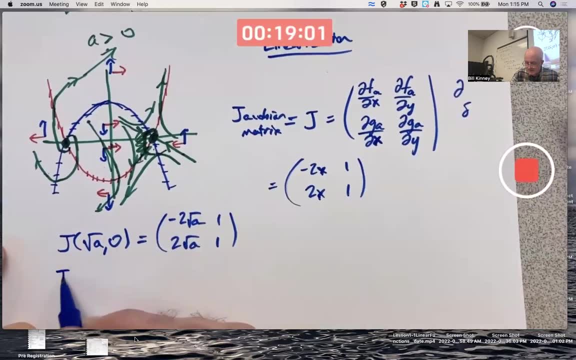 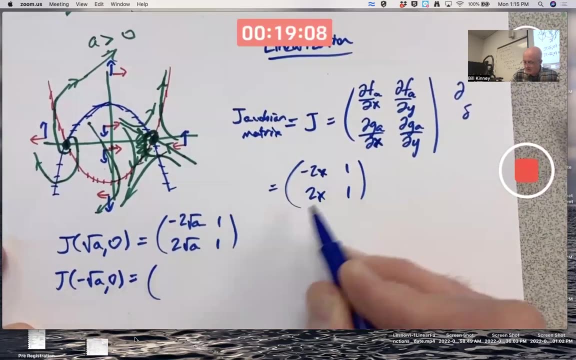 worry about that. there's the jacobian matrix evaluated at the right equilibrium point. if i evaluate it at the left equilibrium point i'm going to have to plug in the equal of room points like a negative square root of a. i get positive two root a. the negative sign just switches where. 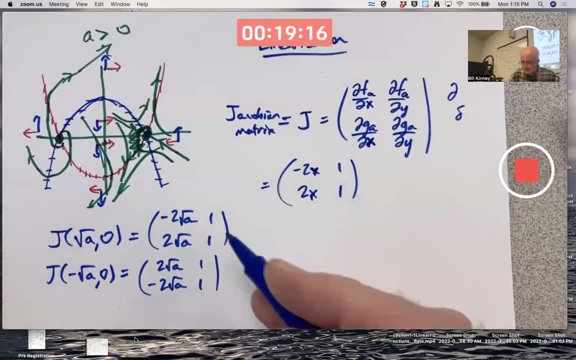 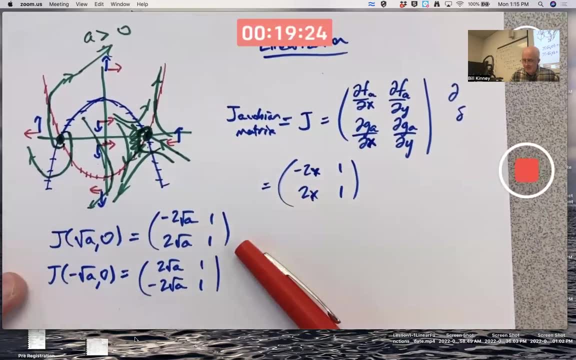 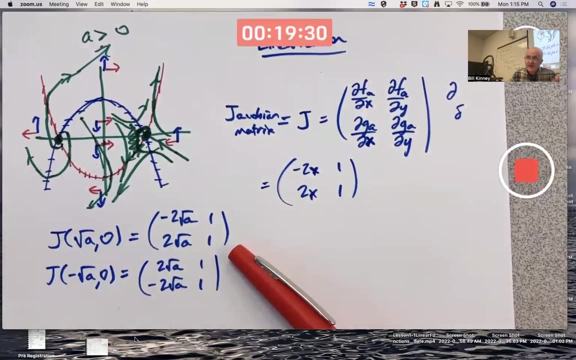 it is, which you might not think is a big deal. you know, is it a really a big difference between these two matrices? just switching the negative sign, it actually does make a big difference. these are two matrices and if a is constant, they are constant matrices, and i could think about the linear system. 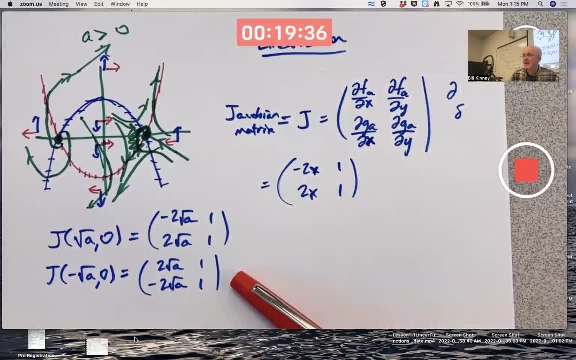 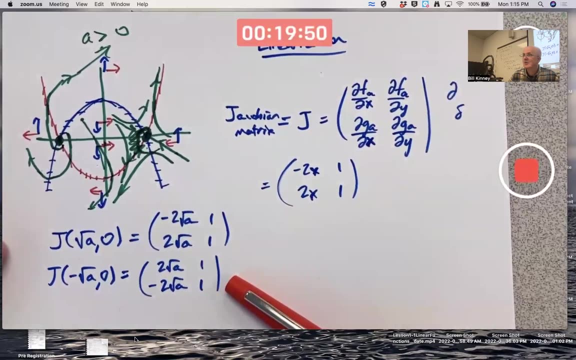 for these matrices. i could think about eigenvalues and eigenvectors, i could think about phase planes, where these are the matrices for my system, and if i'm trying to think about such systems as quickly as possible, the quickest method is to think about the trace determinant plane. 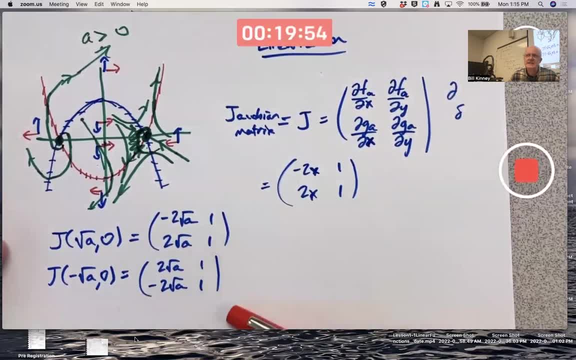 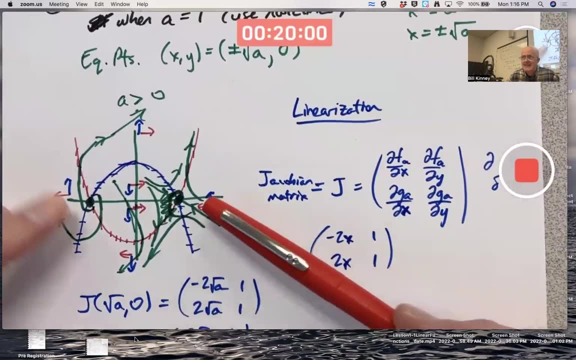 to identify the nature of the equilibrium point at the origin of these systems, at the origin. but wait a minute. the origin is not an equilibrium point. yeah, it's not an equilibrium point for the non-linear system, but i could think about the origin being the equilibrium point for 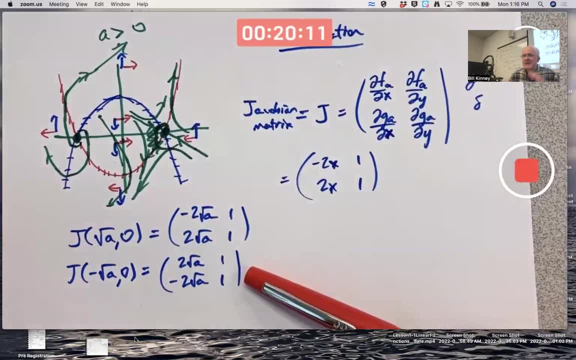 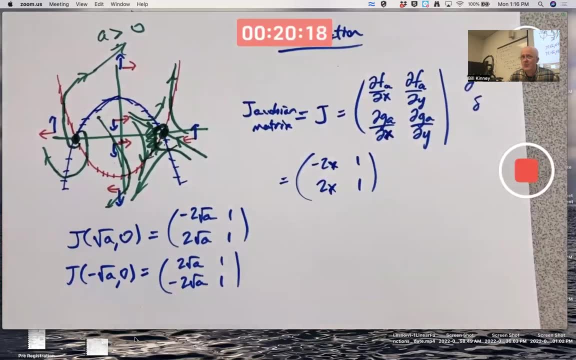 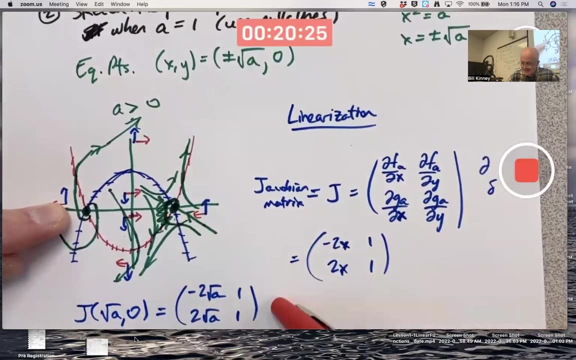 systems corresponding to these matrices and the idea- the big idea here is those systems which are linear, systems where eigenvalues and eigenvectors are relevant- tell you the nature of the equilibrium points for the non-linear systems. we should get this one to be a saddle point and this one to be a spiral source. the trace determinant plane is the quickest way to see that. 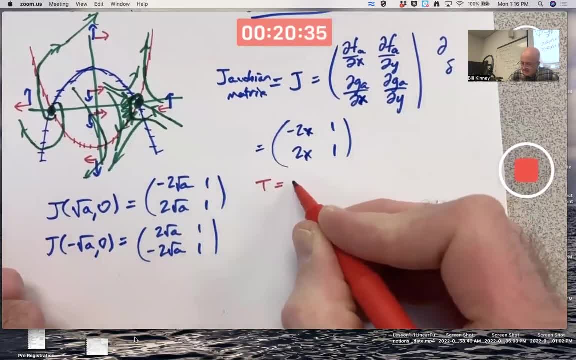 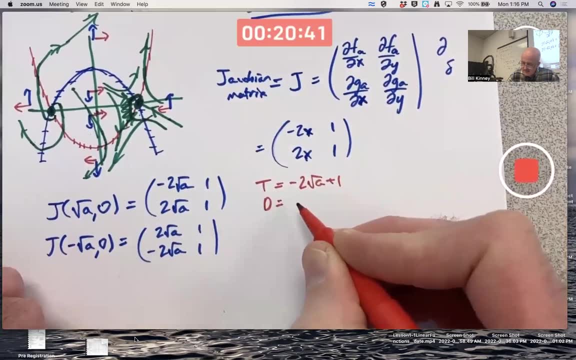 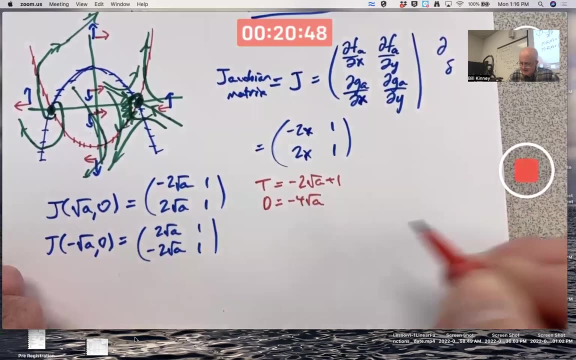 this matrix has a trace of negative two root a plus one and a determinant of looks like it would be minus four root a. all right, double check that in your head. this one has a trace of plus two root a plus one and a determinant of positive four root a. 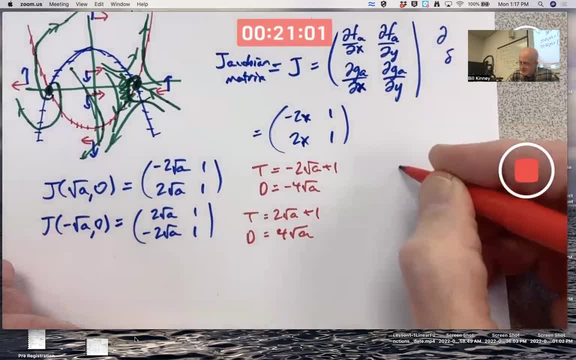 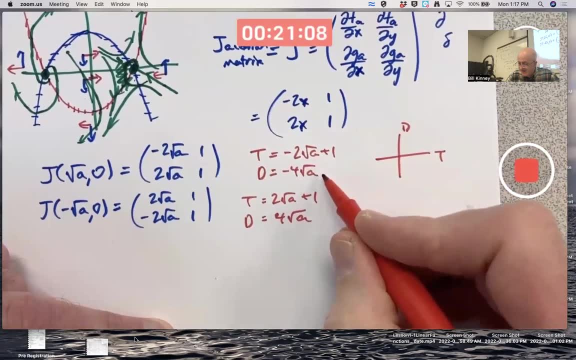 okay, think about this matrix as a spiral source, and it's going to be a spiral source and it's going to be a spiral source and it's going to be a spiral source. the trace determinant plane for this one, no matter what a is, as long as it's positive. 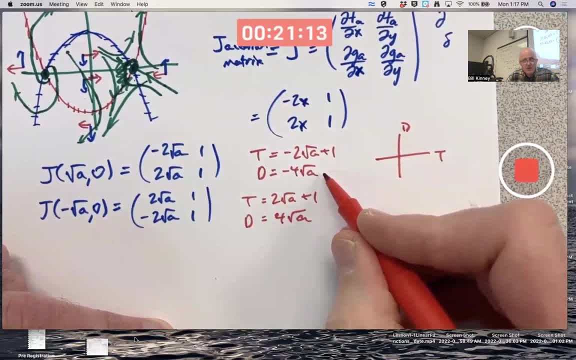 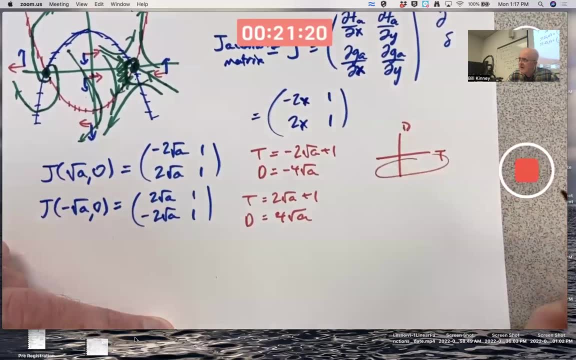 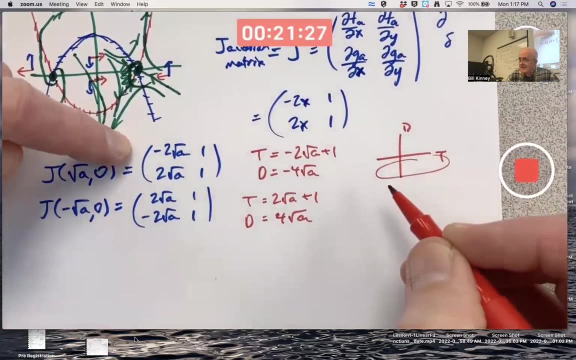 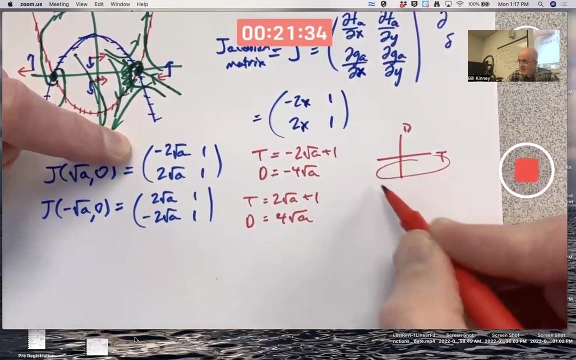 so you're not taking a square root of a negative number. no, no imaginary numbers. here the determinant is negative. you're down here somewhere, meaning for the linear system corresponding to this matrix, the origin is going to be a saddle point. right, that's where saddle points occur. when you're tracing determinant, when you 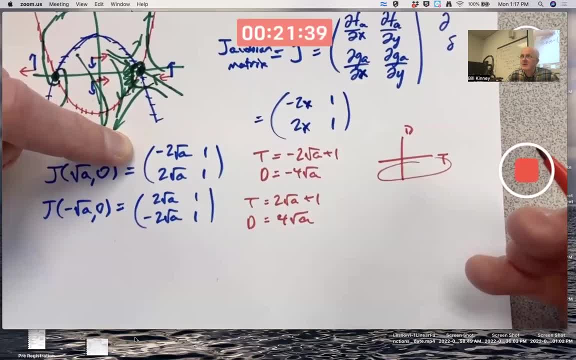 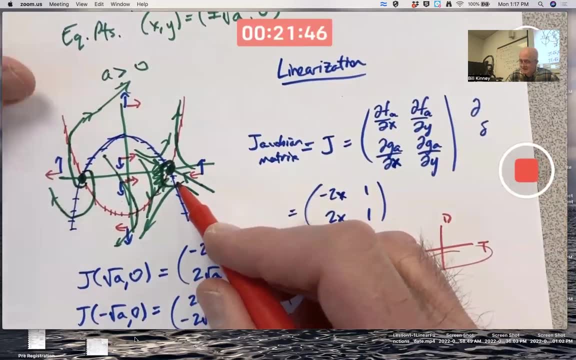 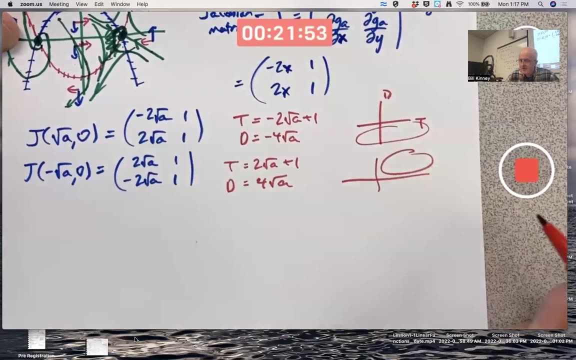 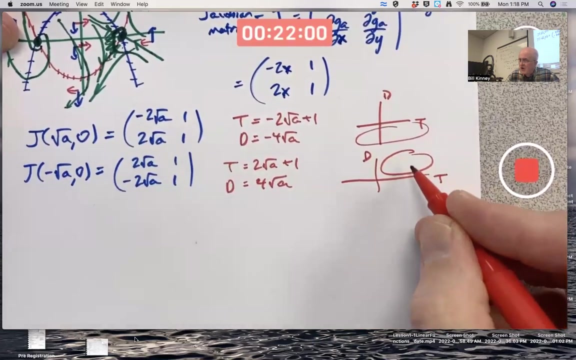 when your determinant is negative, you have a saddle point at the origin, just like this seems to be a saddle point. on the other hand, with this one, the determinant is positive and the trace is positive. you're up here for sure. it's a source. is it a spiral source or a real source? 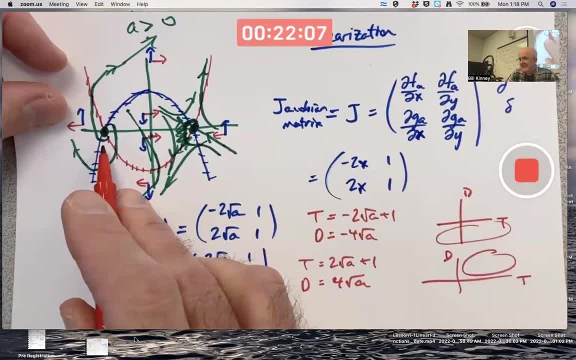 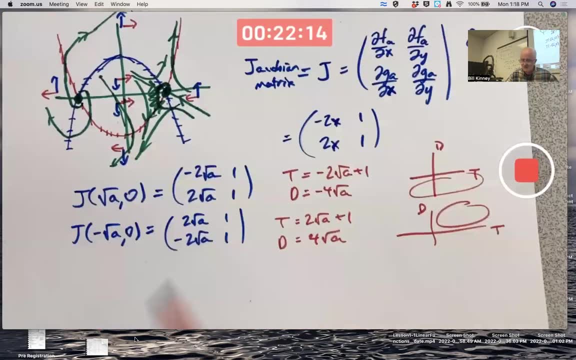 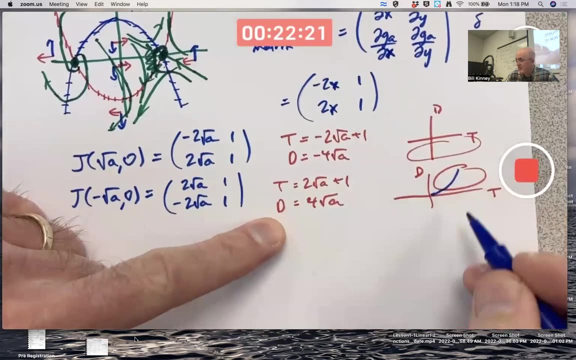 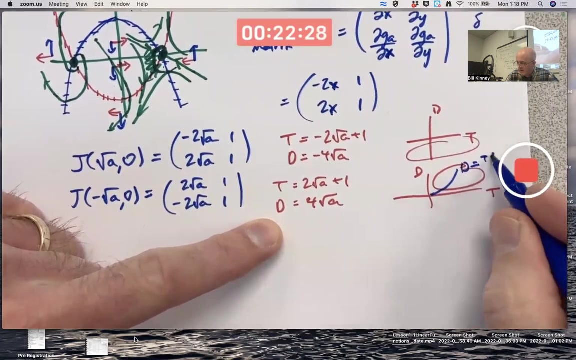 seems to be a spiral source, but maybe looks could be deceiving. is there a way to know for sure? you could think about where the repeated root parabola is here and try to figure out. are we above or below that repeated root parabola? again, that had equation d equals t squared over four. 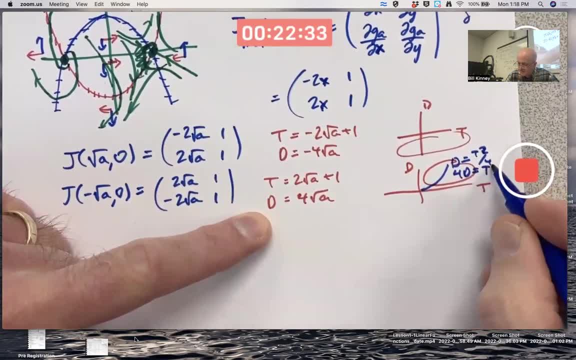 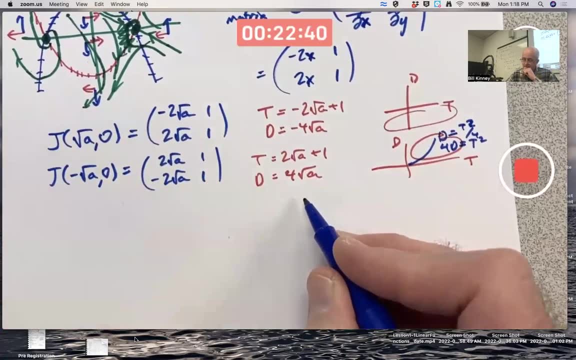 which is equivalent to four. 4d equals t squared. If I calculate t squared and I also calculate 4d, am I going to be above or below the parabola? Is it going to be clear that one of these is bigger than the other? 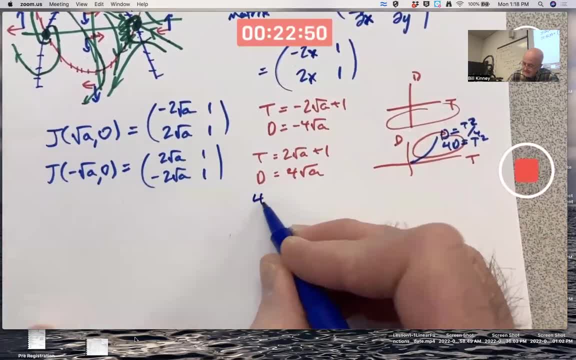 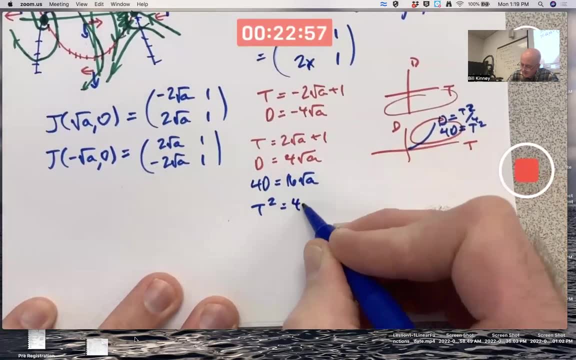 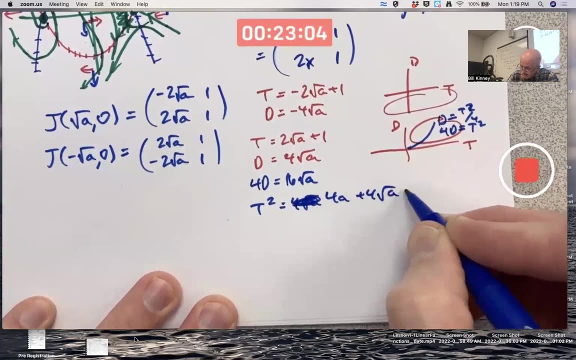 It's not clear to me. 4d is 16 square root of a. What about t? squared? Square that thing. I'll get 4 square root of a. No, excuse me, 4a plus 4 square root of a plus 1.. 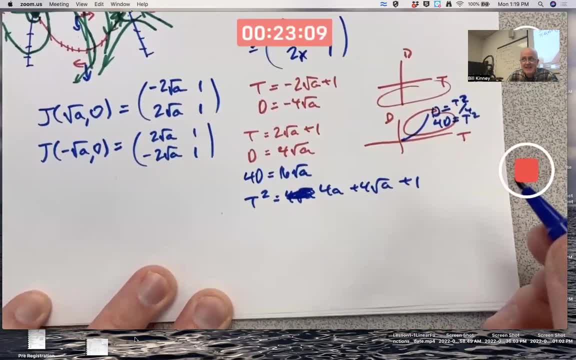 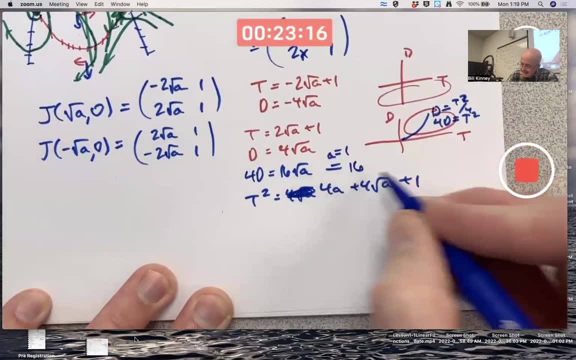 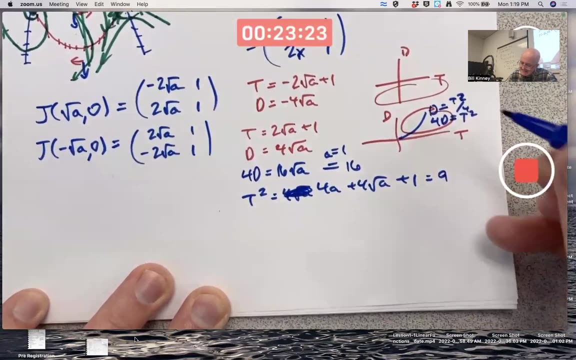 Maybe the answer depends on a. If a is 1,- let's assume we're in the case where a is 1, this becomes a 16 and this becomes a. what 9?? 4d is bigger than t squared. d is bigger than t squared. 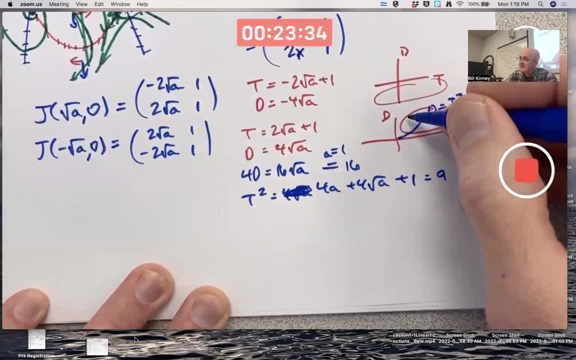 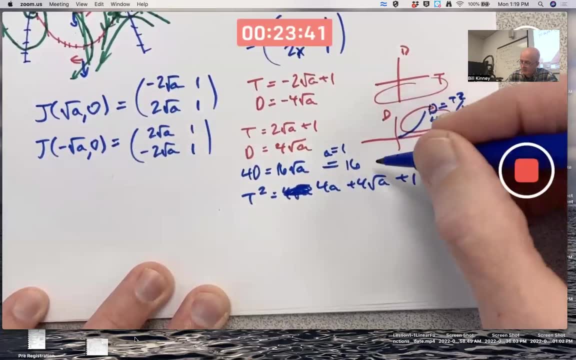 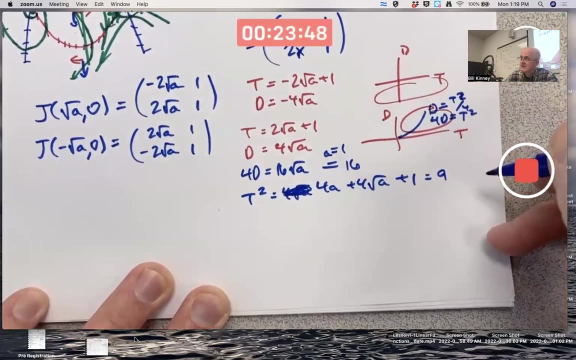 You're above the repeated root parabola. Spiral source: when a is 1, at least 4d is bigger than t squared means d would be bigger than t squared over 4.. You'll be above that curve, Just like it looks like a spiral source. 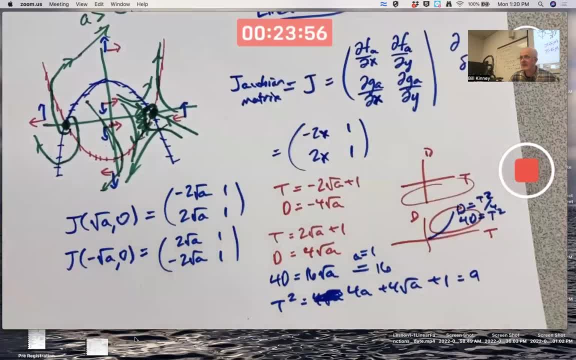 Technically speaking, what's going on here in justifying all this is something called the Hartman-Grobman theorem, which I do Talk about in the lectures. It's a very, very advanced theorem, Very difficult to prove. We do not prove it in any, we do not even come close to proving it. 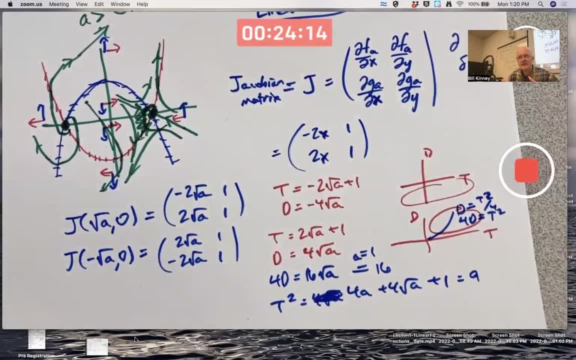 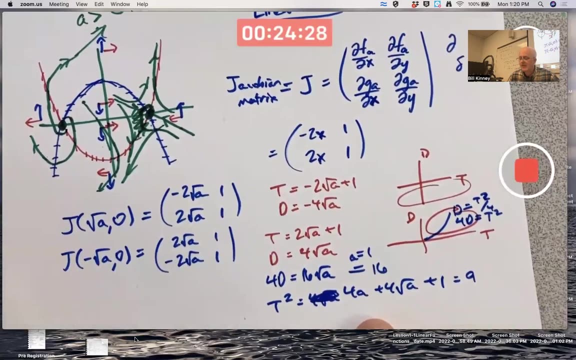 We do not even come, we don't even really fully use it, We just sort of talk about it to get a little intuitive feel for what it means to justify such a thing, The fact that we're not on the positive dx, Yeah. 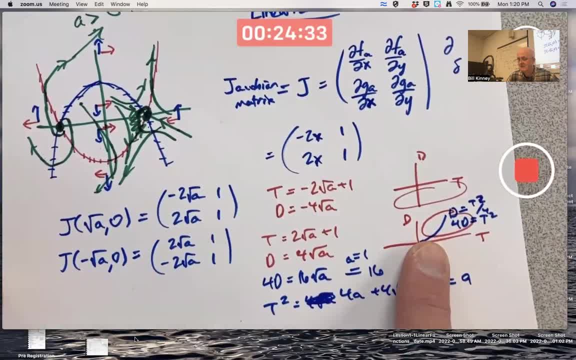 The fact that we're not on the positive dx is actually important, Although, in fact, if a is 0,, if a is 0, then okay, never mind. If a is 0,, the determinant is 0, and the origin is kind of a degenerate equilibrium point. 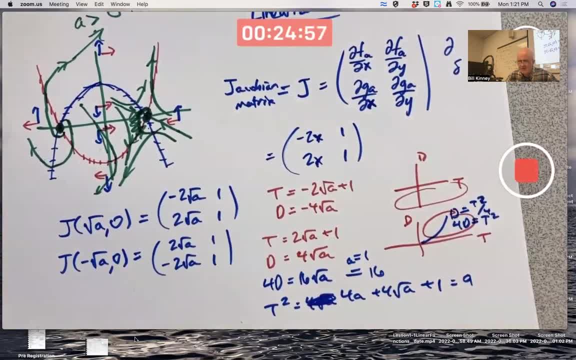 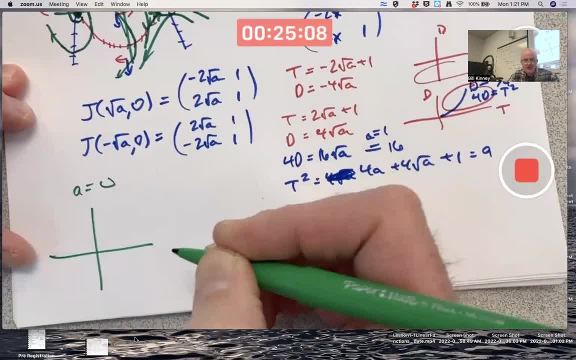 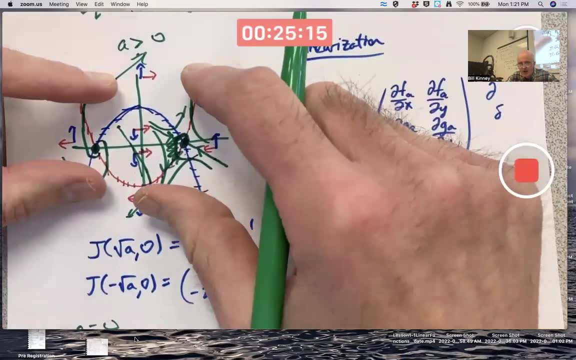 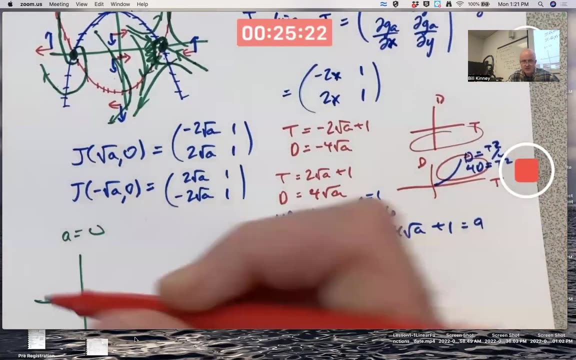 I'm not going to do a full analysis here As a increases towards zero or decreases towards zero, So I'm imagining a decreasing here. These parabolas are going to merge. Well, they don't literally merge, They, they, they move together, so to speak, so that these points move toward the origin. 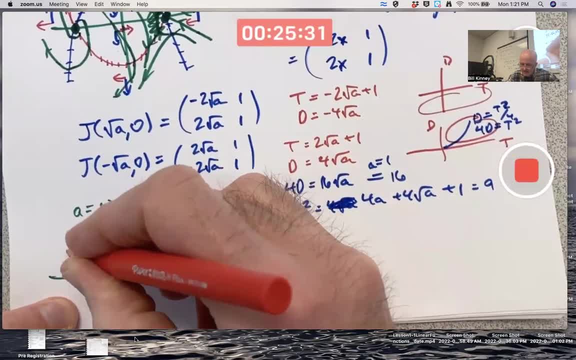 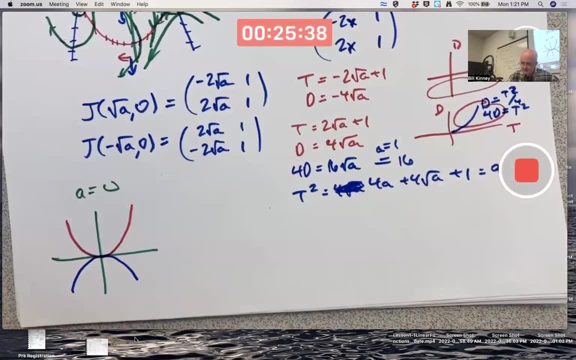 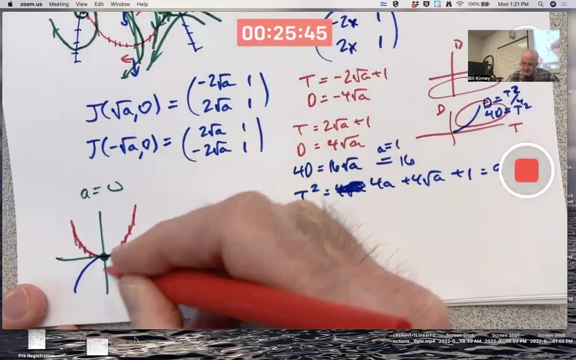 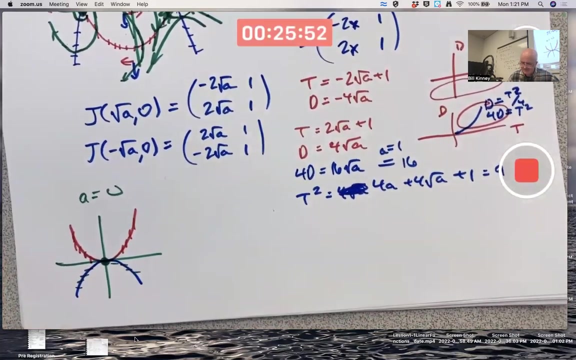 The red one becomes this one when a is zero and the blue one becomes this one. You've got one equilibrium point at the origin. Still crossed the red one vertically and the blue one horizontally. Do I want to bother? Let's not bother doing this by hand anymore. 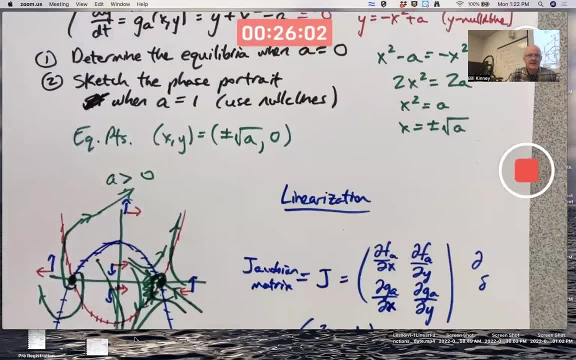 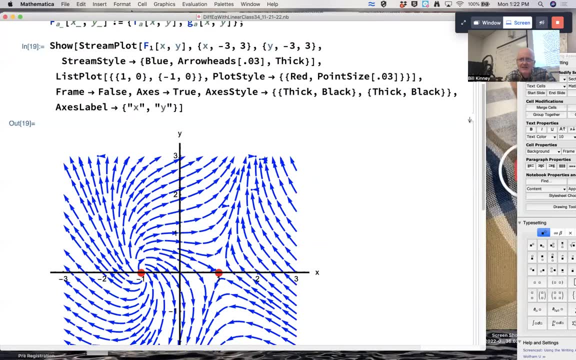 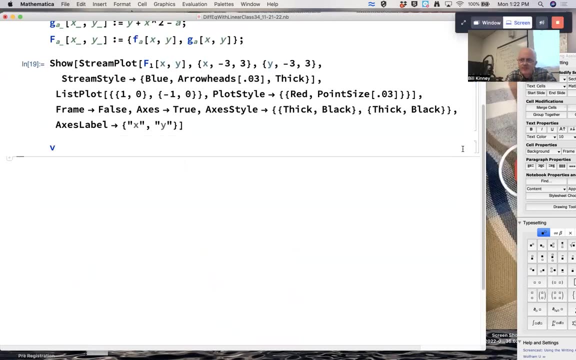 because I want to do something else. Let's quickly look and see what Mathematica produces. So here's Mathematica's stream plot when A is 1.. But I want to see what happens as A changes here. I could put this inside and manipulate. 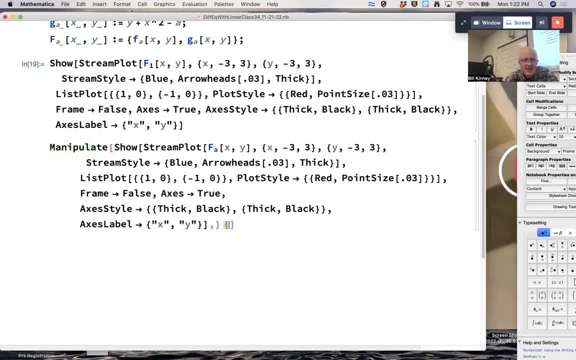 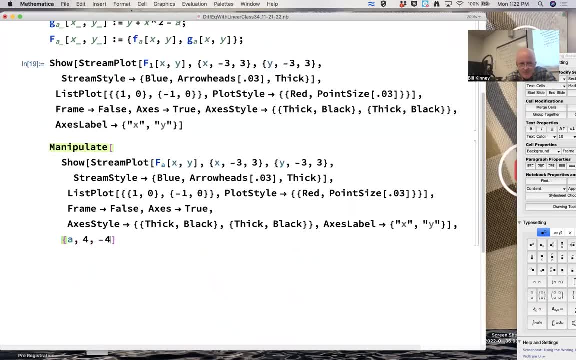 And change this 1 to an A, And let's actually let A decrease. So I'll start with A, to be, say, 4, and go down to negative 4.. That'll make A decrease. Those equilibrium points are in the wrong spot, though, then. 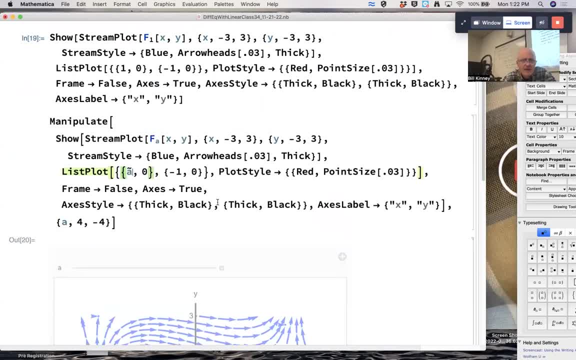 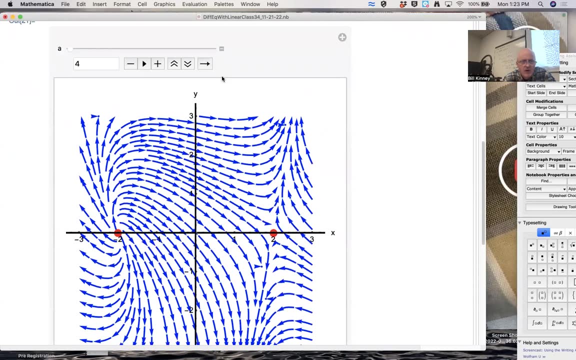 Let's see here Square root of A, Oops, Square root of A, and negative square root of A. So watch what happens as A decreases. So here A is 4.. Two equilibrium points, A bigger value of A- I'm looking at this. left one. 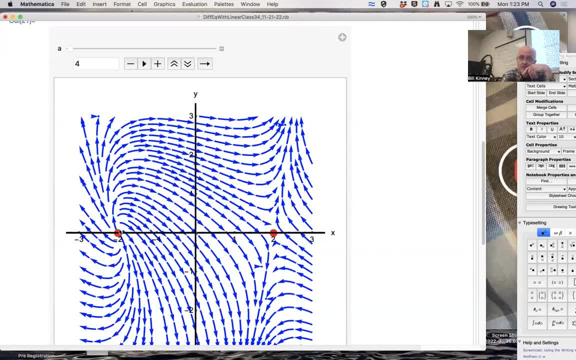 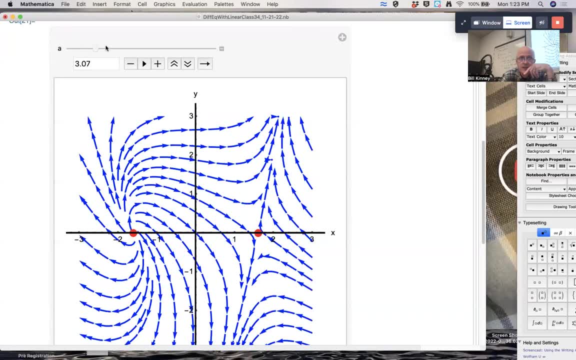 It looks like. maybe it's more likely to be a non-spiral source there. If A is big enough, As A decreases towards 0, like when it's 1, does it more clearly become a spiral source. See, it's looking more and more like a spiral source. 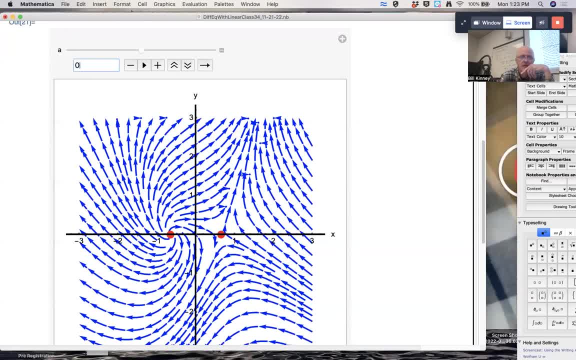 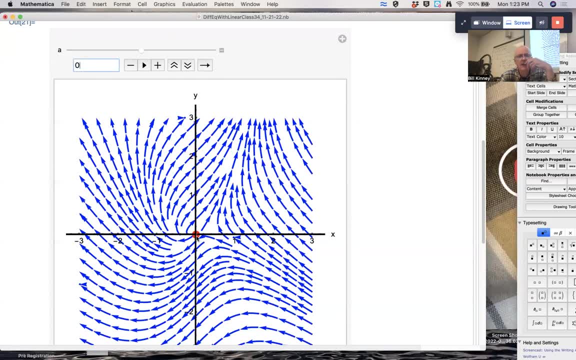 When A is 0, it's a non-spiral source. The equilibrium points have merged. What kind of behavior is it near the equilibrium point at the origin? It's kind of weird actually. It's like it's half of a spiral source and half a saddle. 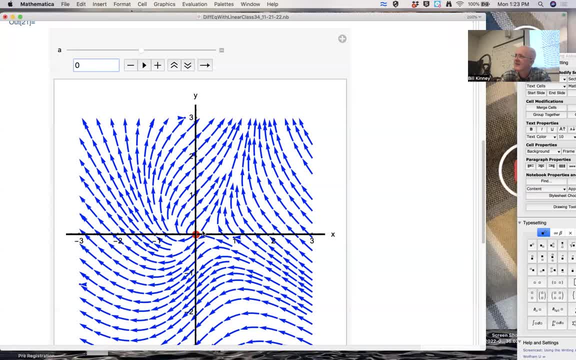 Isn't that weird? Is that really what's going on? Yeah, it actually is. It's called a degenerate equilibrium point in that case, And linearization doesn't work anymore. So what happens when A is 0? When A is 0,? 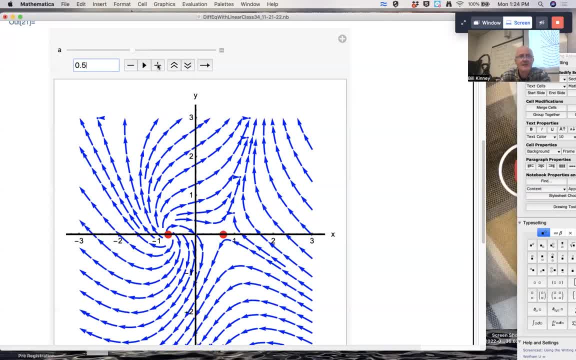 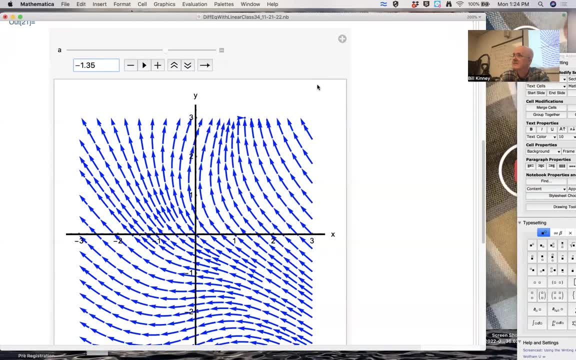 when A is negative, then Why is it going backwards? When A is negative, there's no more equilibrium points, So a bifurcation has occurred. It's like the equilibrium points are matter and antimatter. They've come together, They've annihilated each other. 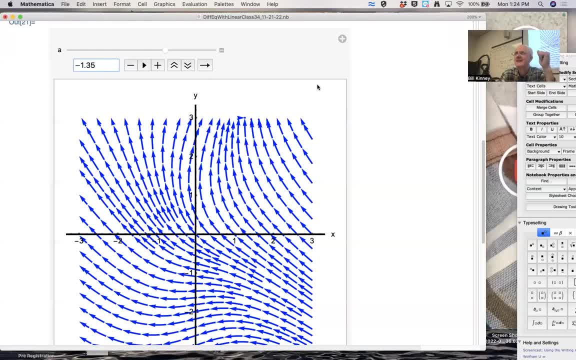 Is that really an application? No, it's just for fun. Okay, It's just pretend. Okay. 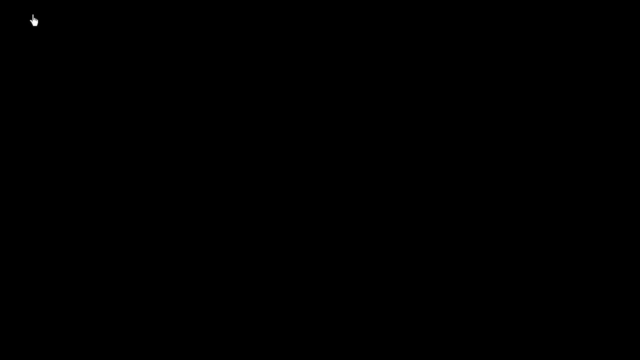 We've been talking a lot about infinite series and now we're going to talk about using infinite series to actually define functions, And the most common infinite series used to define and approximate functions is a power series. So I could have a function f of x defined. 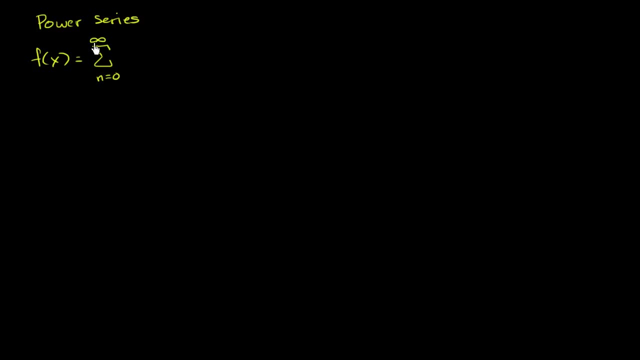 as the infinite series. so we'll go from n equals 0 to infinity of a sub n times x minus c, to the n-th power, where a sub n is just the n-th coefficient and c is some constant and x, of course, is our variable. 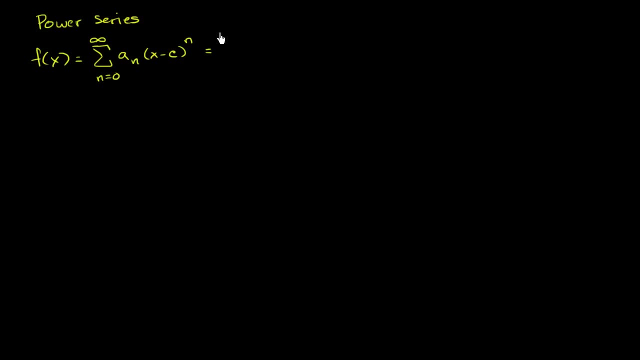 So this right over here is a function of x, and it might be a little bit clearer if I expand this out. This is going to be our 0-th coefficient times x minus c to the 0-th power, which is, of course, this part is just. 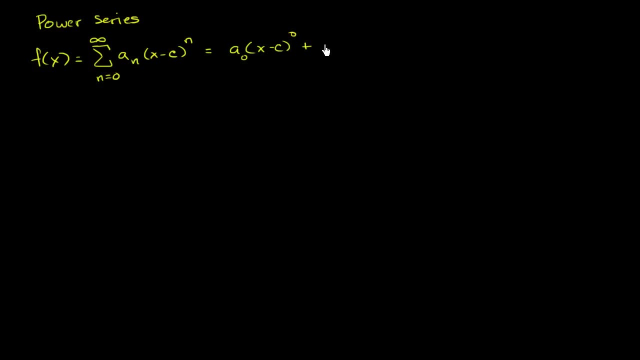 of course equal to 1, so this would simplify to a sub 0, plus a sub 1.. Times x minus c to the first power, plus a sub 2 times x minus c to the second power. And we could go on and on and on.